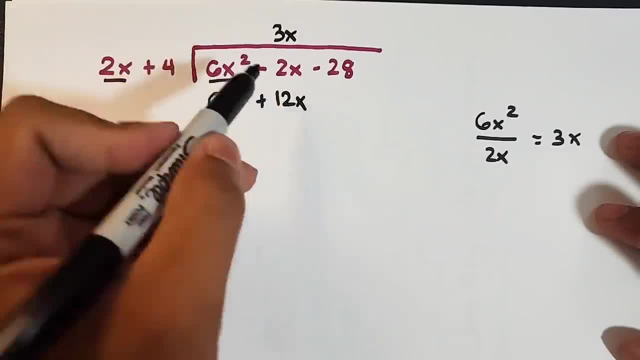 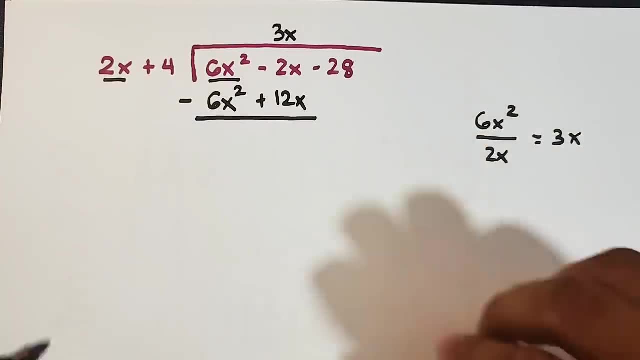 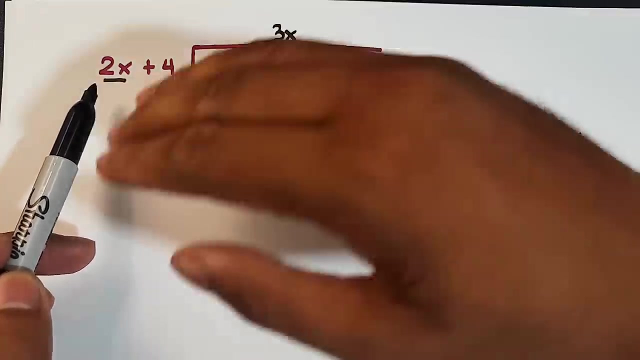 12x. So we know that, after multiplying, we have to subtract. So that's it, Guys. it's just a rotation. The first thing we do is we divide the leading terms And then, after dividing, multiply And then, lastly, subtract. This is our rotation. 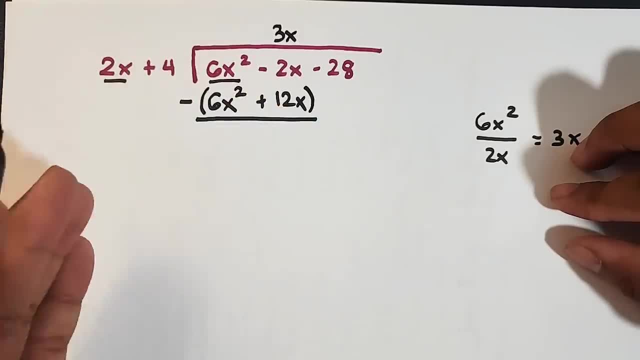 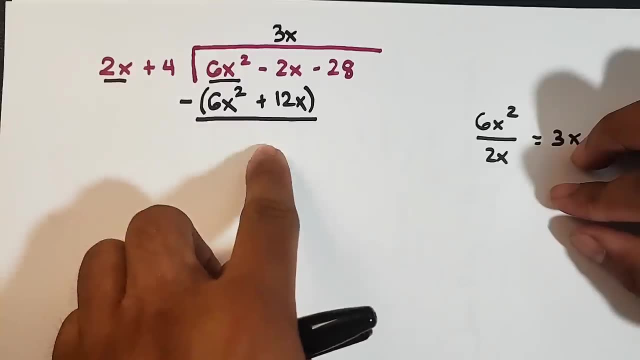 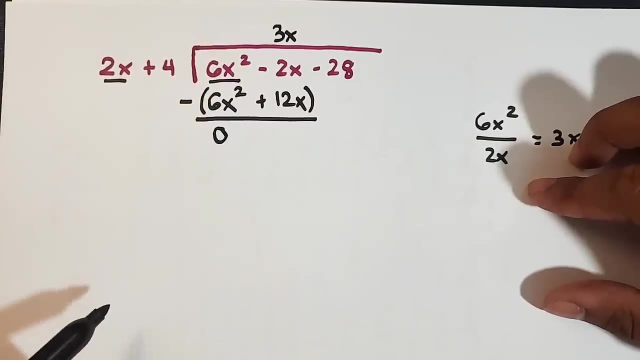 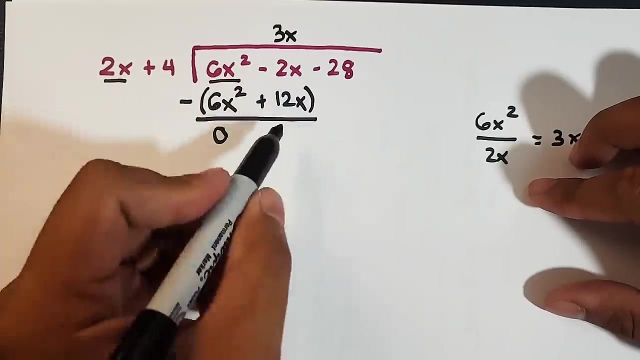 Include the parentheses here so you won't make a mistake. Always enclose by the parentheses. by parentheses, The answer to multiply Okay. So that is 6x squared minus 6x. If you will notice, it will be zero, Okay, Zero. And then here our negative 2x minus 12x, it will become 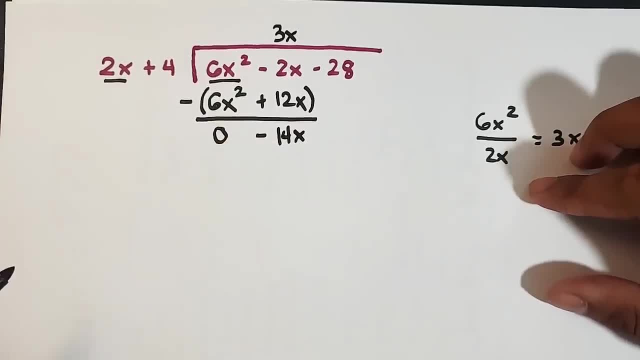 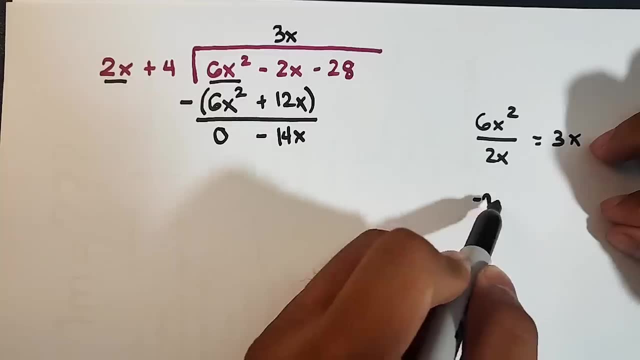 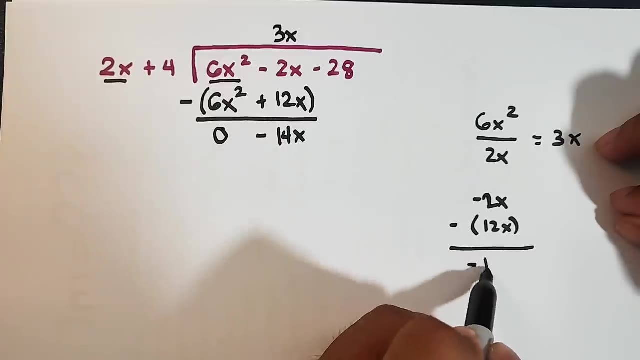 negative 14x. Wow, Okay, Okay. So what happens here, guys? I'll just show you Negative 2x minus 12x. This 12x will be negative. It will be negative 2x. 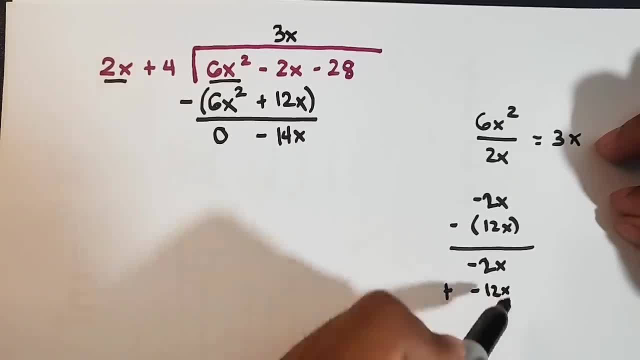 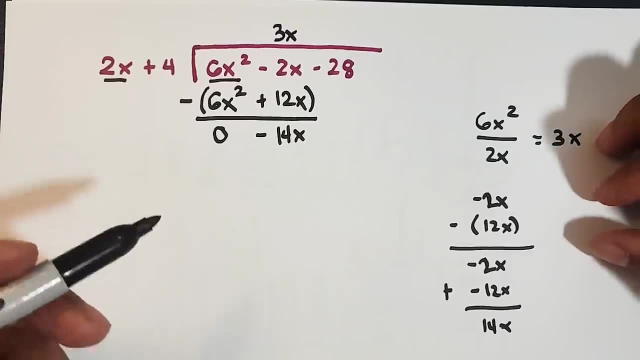 Then it will be plus this, plus negative 12x, So they will be the same sign. So we'll add this. The tendency will be 14x. Okay, Let's continue here. So we have negative 14x. 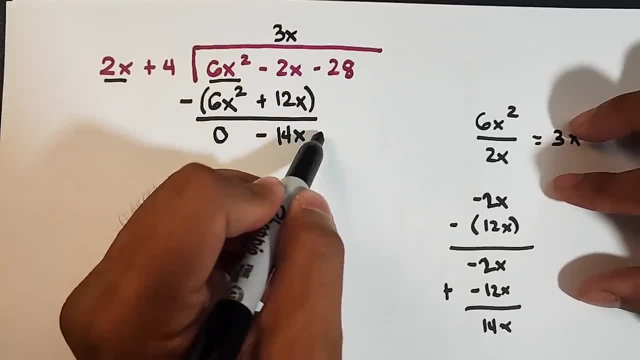 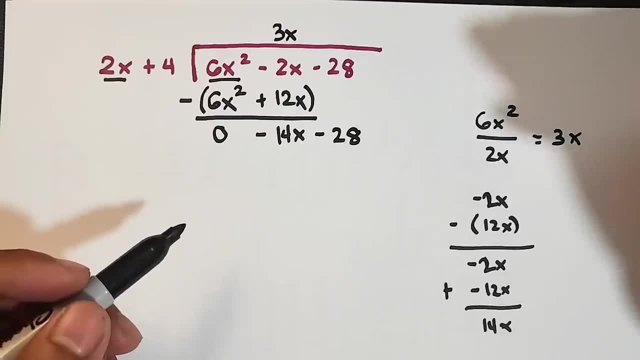 Then, after that, you will bring down negative 28.. So negative 28.. Now what's next? This is your new dividend. So same rotation, Let's divide. Let's divide the new leading term, which is negative 14x, by the leading. 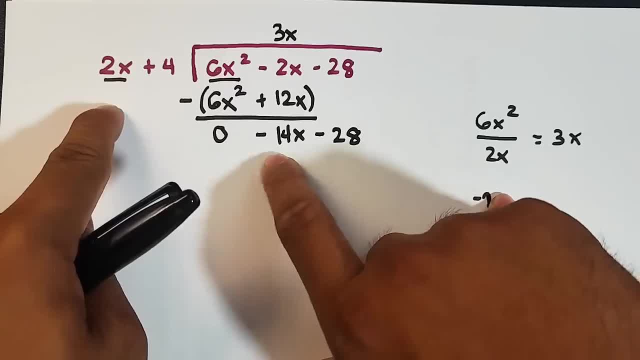 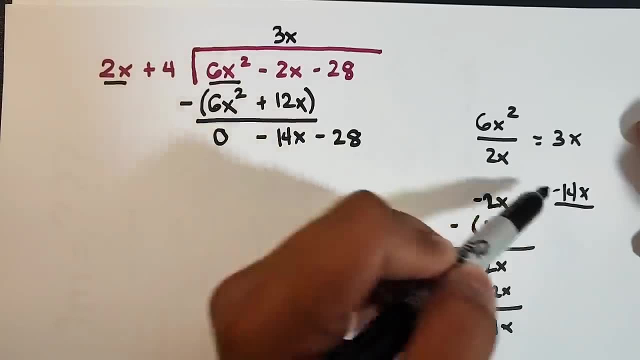 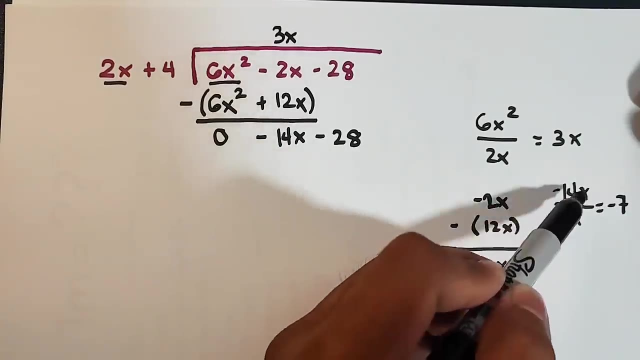 term of your divisor. Okay, So we have negative 14.. I will use this part: Negative 14x divided by 2x 2x. So negative 14 divided by 2 is negative 7.. And then x over x. 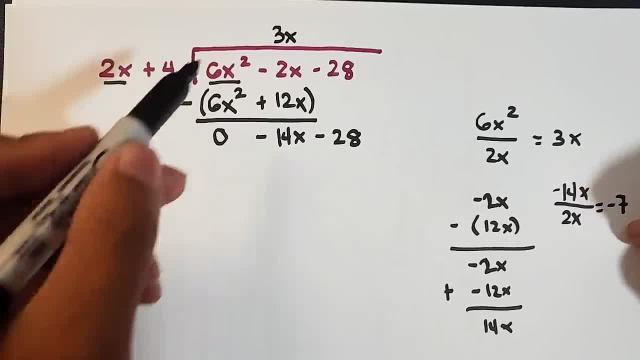 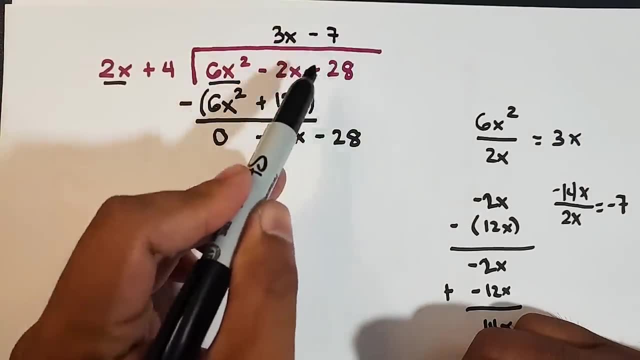 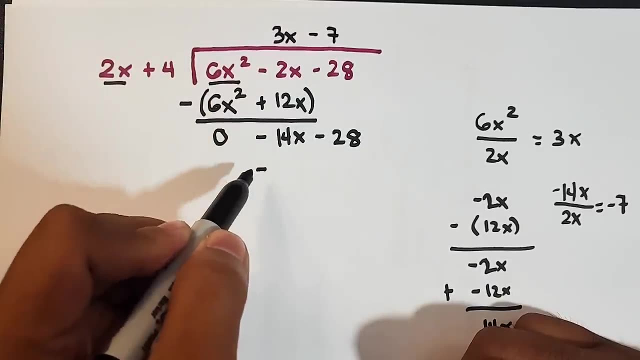 is 0, or 1.. So negative 7.. So this will become minus 7.. Okay, So what we have here after dividing: multiply again: negative 7 times 2x, That is negative, negative. 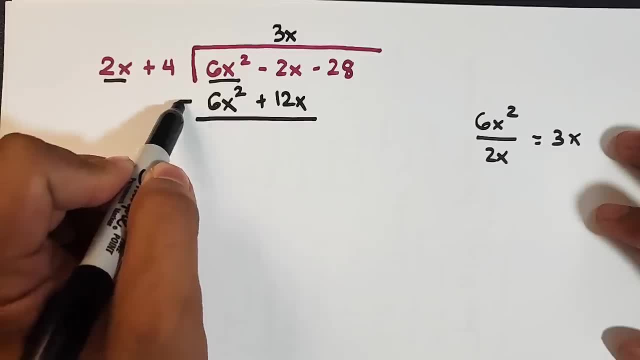 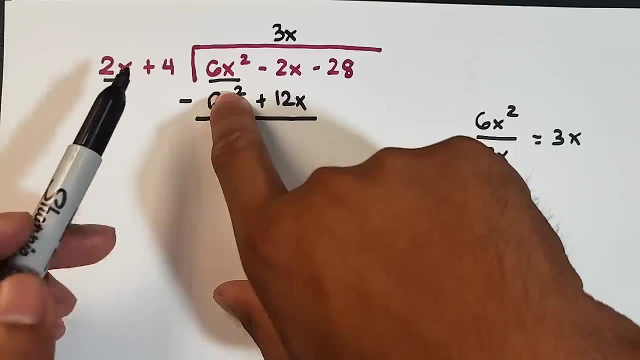 So we know that after multiplying, we have to subtract. So that is it, guys. It is just a rotation. First we divide the leading terms And then, after dividing, multiply And then, lastly, subtract. This is our rotation. 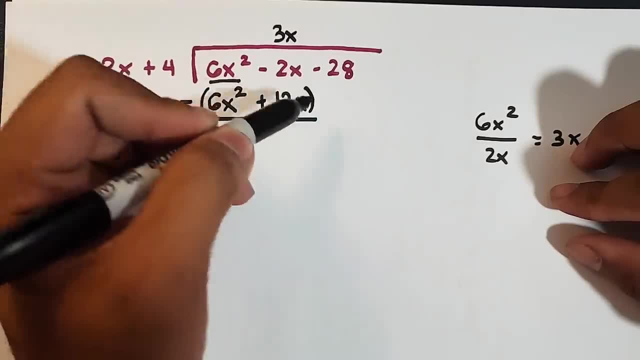 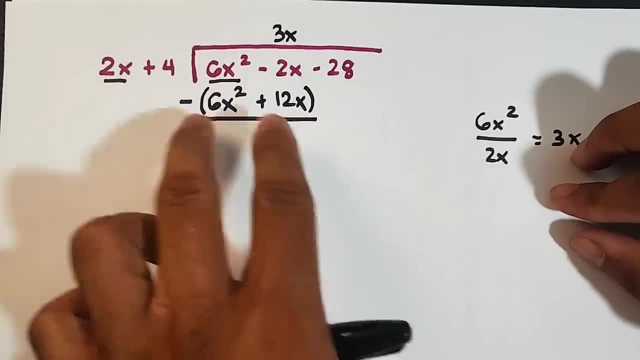 Now Inclose this in parentheses, guys, So you won't make a mistake. Always enclose by parentheses The answer you got in multiplying. Okay, So that is 6x squared minus 6x. If you notice, it is 0.. 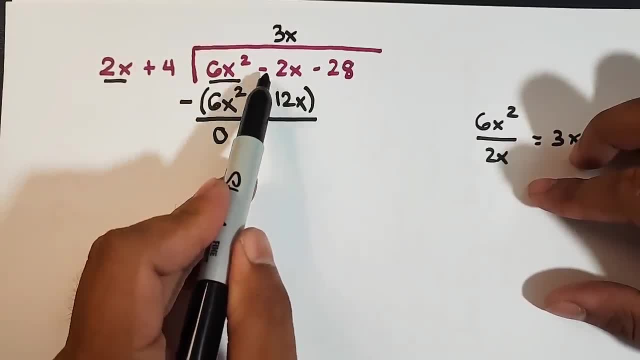 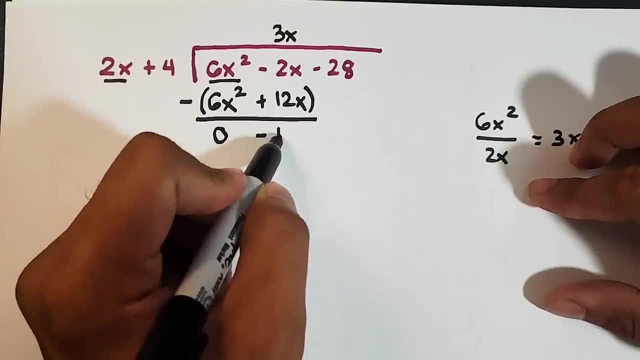 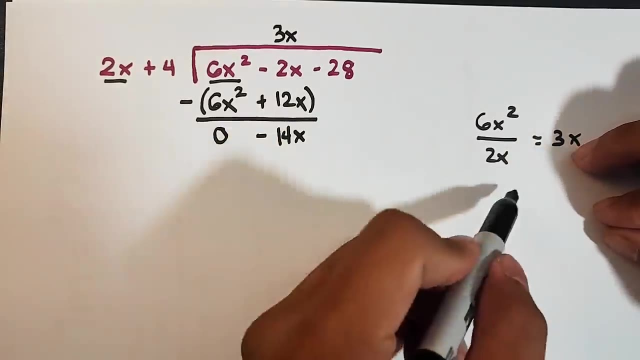 Okay, 0.. And then here our negative 2x minus 12x, it will become negative 14x. Okay, So what will happen is that, guys, I will just show you Our negative 2x, then minus 12x. 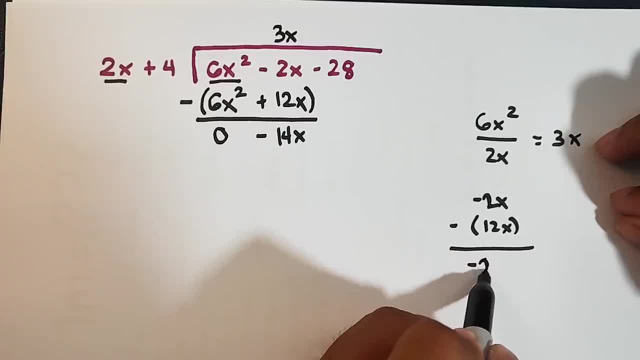 Our 12x will become negative. It will become negative 2x. Then it will become plus 2 plus negative 12x. So the same sign will become the same sign. So we will add this. The tendency will become 14x. 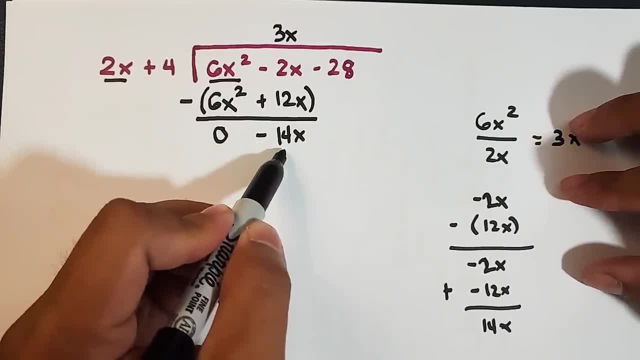 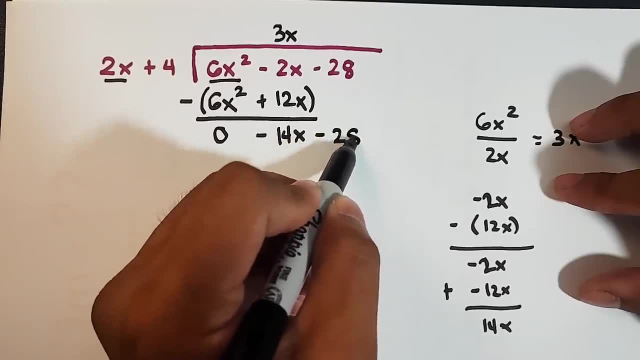 Okay, Let's continue here. So we have negative 14x, Then after that you will bring down negative 28.. So negative 28.. Now what's next? This is your new dividend. So same rotation. Let's divide. 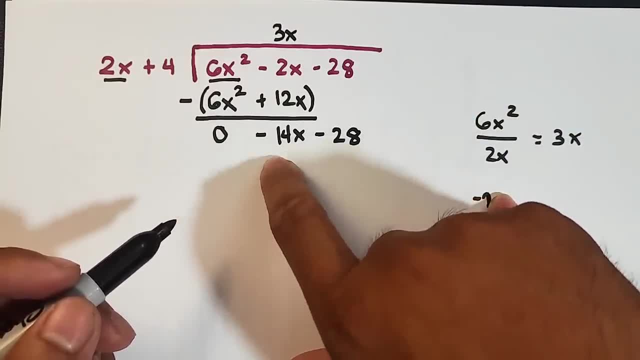 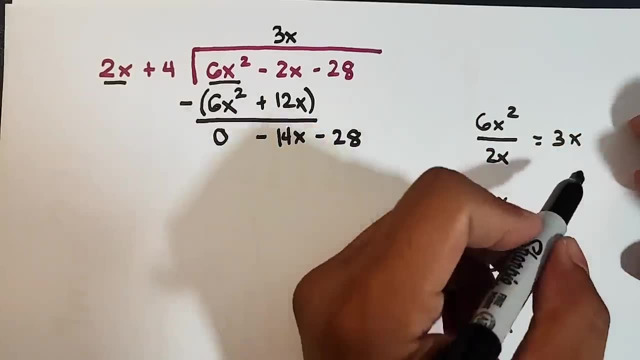 Let's divide. Let's divide the new leading term, which is negative 28.. Let's divide the new leading term, which is negative 14x, by the leading term of your divisor. Okay, So we have negative 14.. I will use this part. 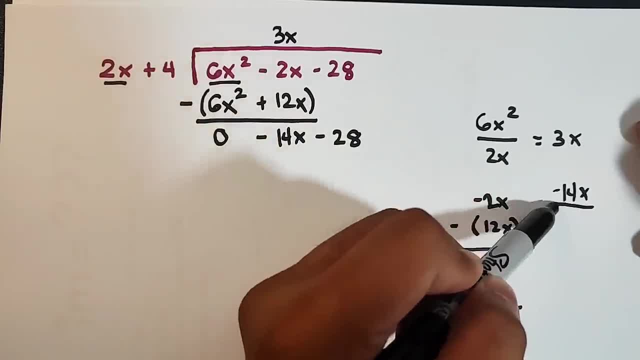 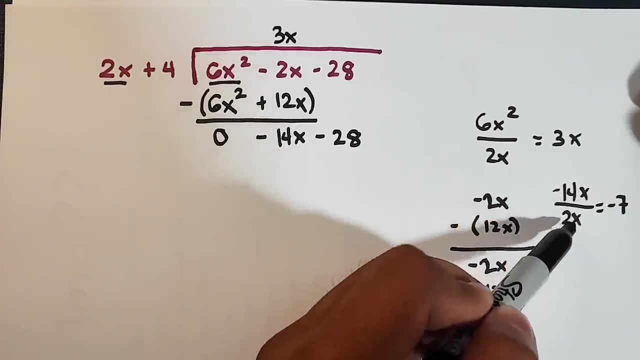 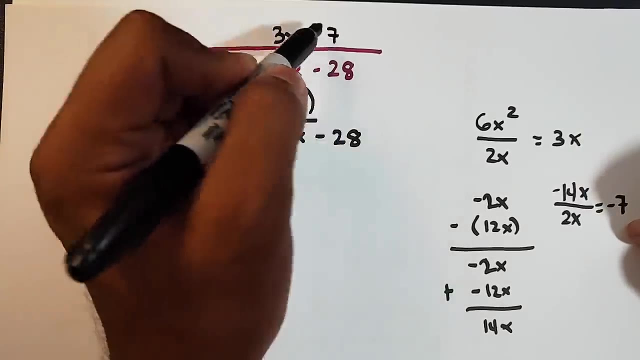 Negative 14x divided by 2x, So negative. 14 divided by 2 is negative 7.. And then x over x is 1.. So negative 7.. So this will become minus 7.. Okay, So what we have here? 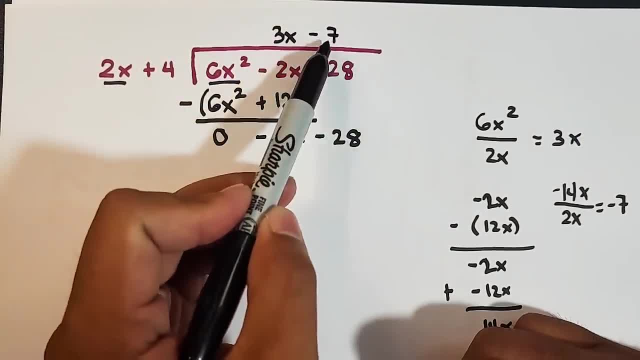 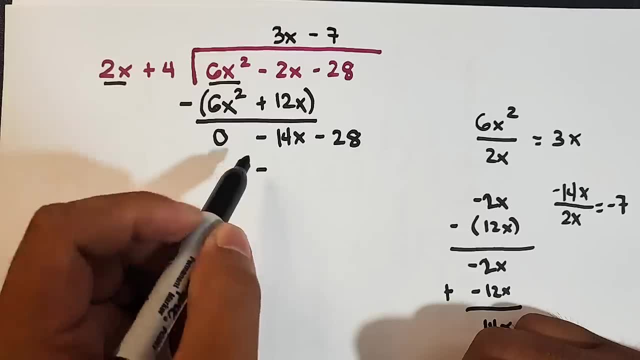 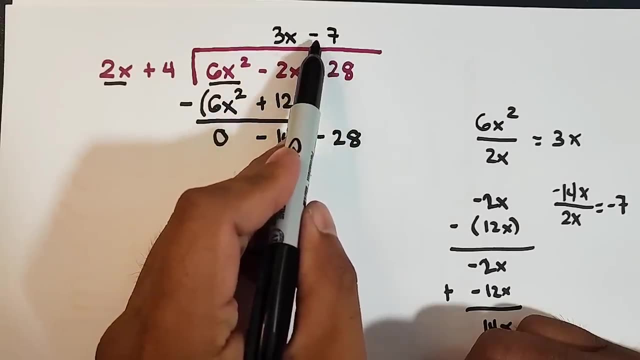 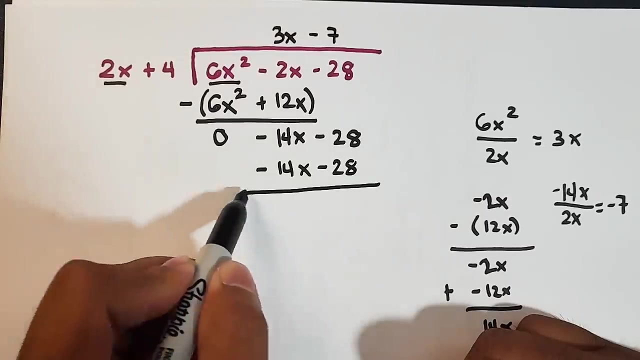 after dividing, we will multiply again. Negative 7 times 2x, That is negative 14x. Next negative 7 times 4.. That is negative 28.. So let's subtract, But you can close it with a parenthesis. 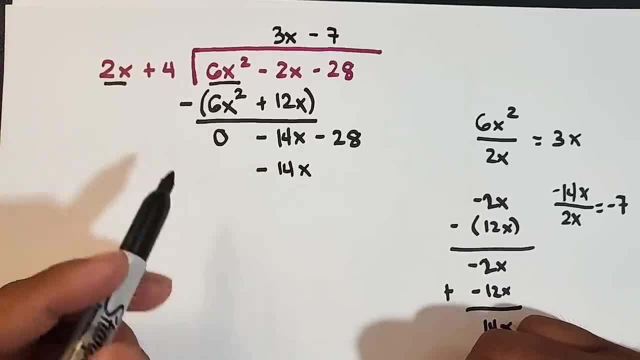 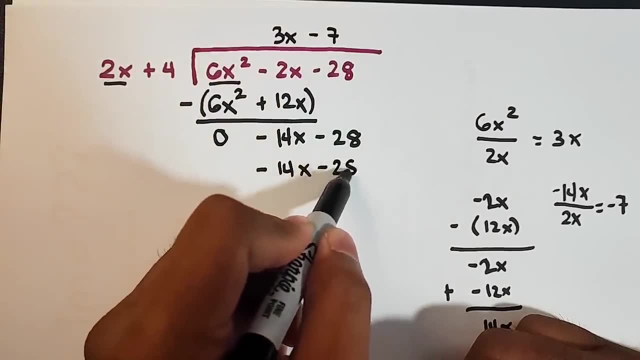 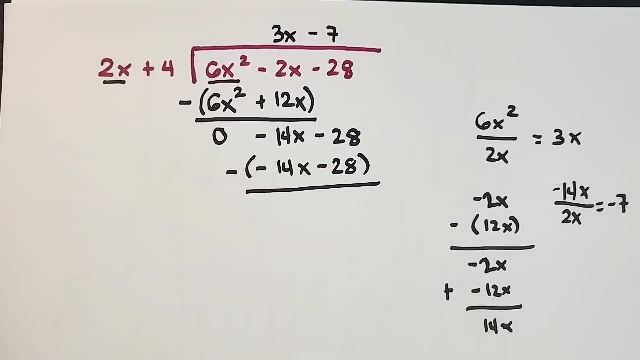 14x. Next negative 7 times 4, that is negative 28.. So multiply natin, Ah, subtract natin. Pero yung close mo sa parenthesis to ah, Eto na, baka malito kayo. 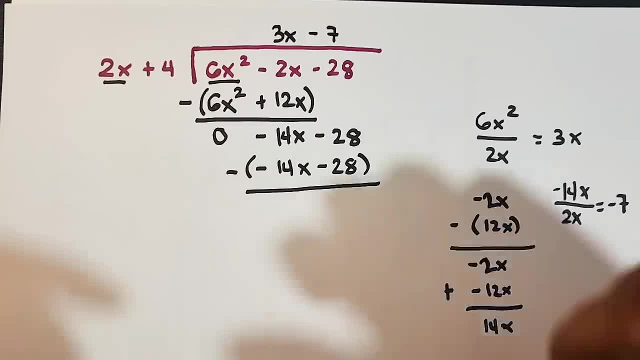 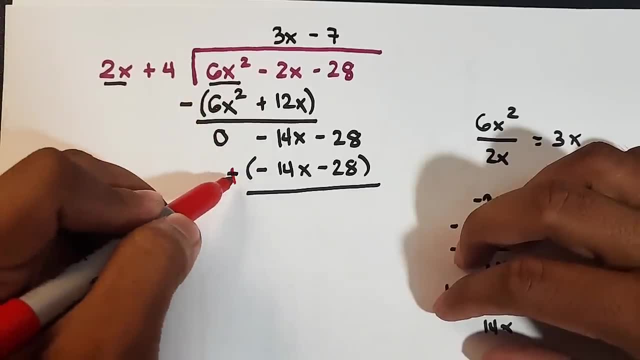 Here it is. You might be confused. What happens here, guys? Here they will change the sign. Here the sign changed, but I didn't see it. But here, this will become an addition. This will become an addition. 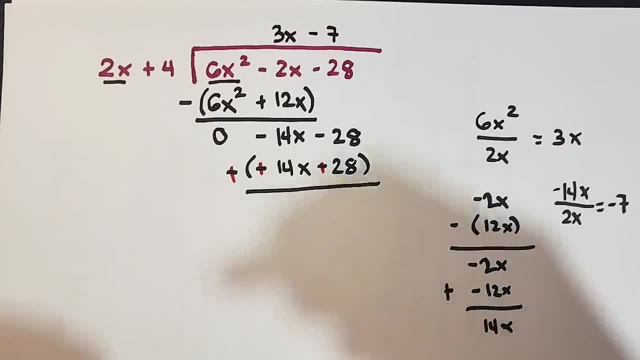 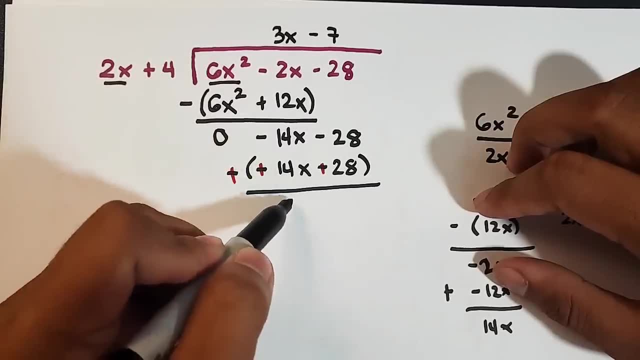 This will become an addition as well. Okay, That is our rule here. So, as you can see, negative 14x plus 14x is already positive, So that is 0.. That is 0.. Negative 28 plus positive 28.. 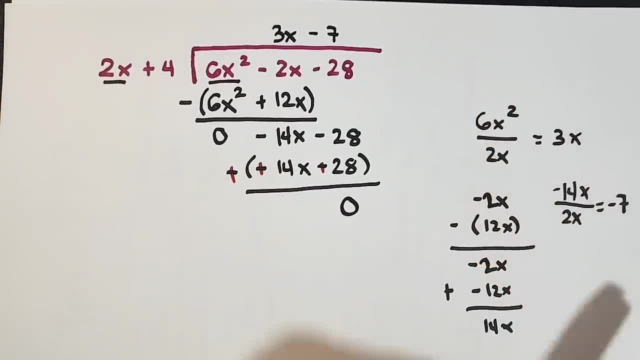 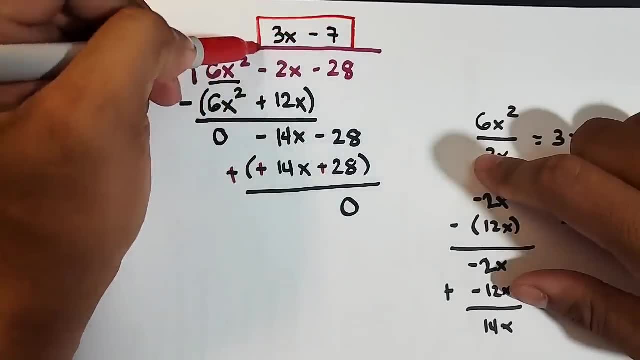 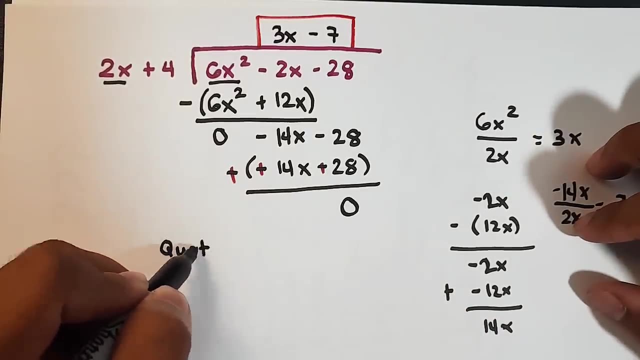 That is 0.. So, after adding 0,- let's stop- It means your remainder is 0.. Again, your remainder is 0.. And the quotient is this: The quotient. Let's add it. The quotient is equal to 3x minus 7.. 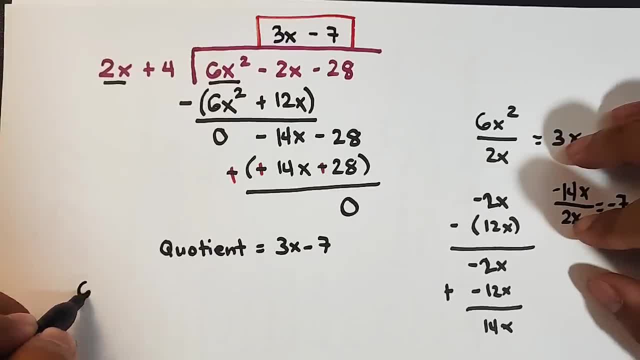 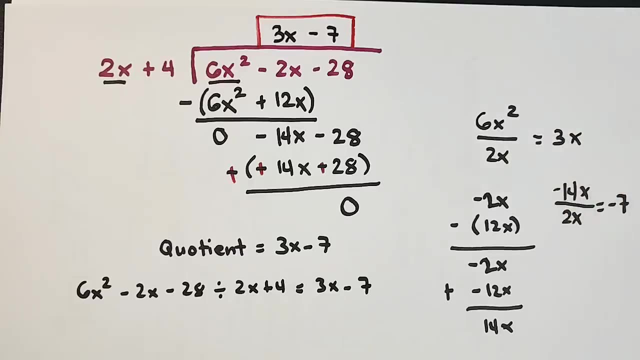 Or what we can do here is that we have 6x squared minus 2x minus 28, divided by 2x plus 4. It's equal to 3x minus 7.. And that's it, guys. So let's continue solving the next problem. 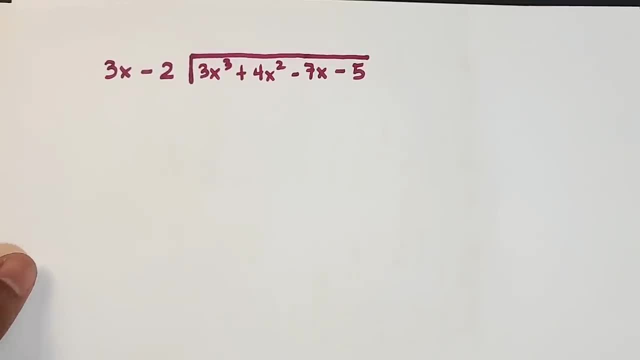 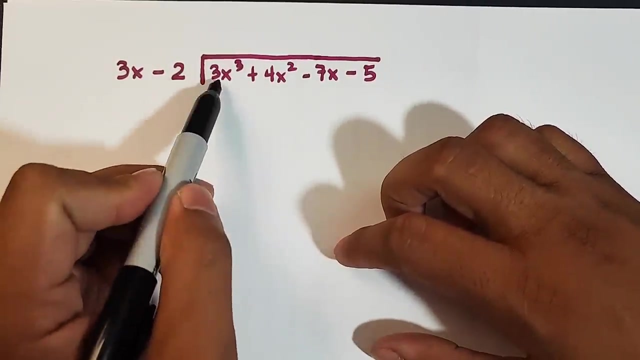 Okay, Let's have another problem. For the next problem, same rotation: Divide the leading terms, Multiply and then subtract, Let's try. Okay, So let's try this one Leading term, leading term: 3x cubed divided by 3x. 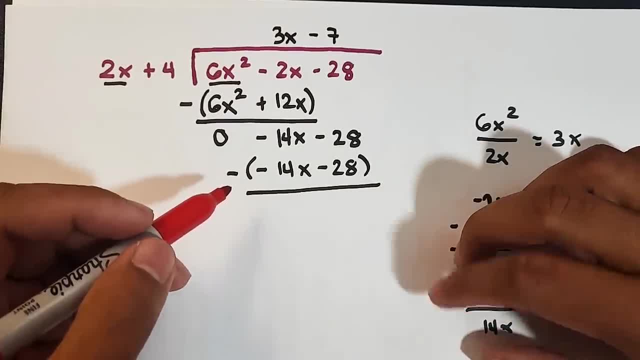 Anong yari, dito guys, Eto ha Magbabago sila ng sign, Dito kasi nagbago ng sign, pero hindi ko na pinakita. Pero dito kasi eto magiging addition, eto magiging addition, eto magiging. 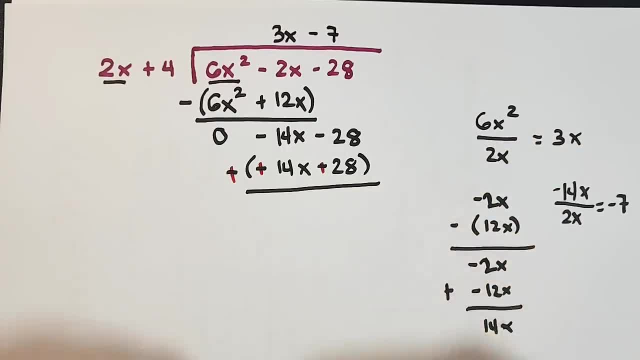 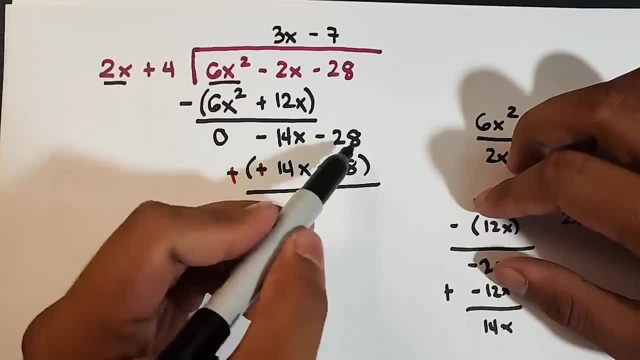 addition din. Okay, Ganun yung rule natin dyan. So, as you can see, negative 14x plus 14x, positive na yan, eh So 0.. 0 na yan, Negative 28 plus positive 28,. 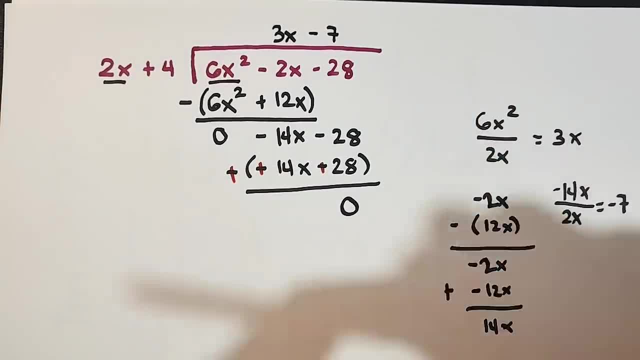 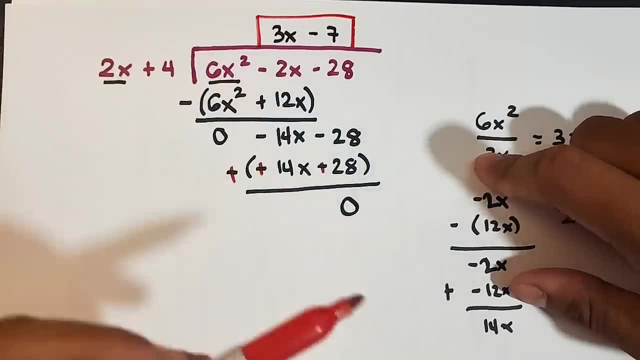 that is 0.. So, pagdaging 0, na stop na tayo. Ibig sabihin, your remainder is 0.. Again, your remainder is 0, and the quotient is this: The quotient dagyan natin, eh. 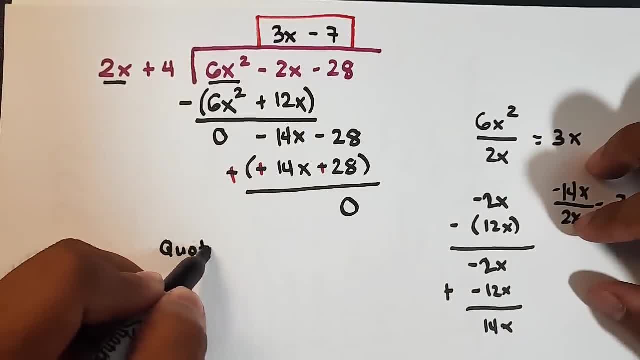 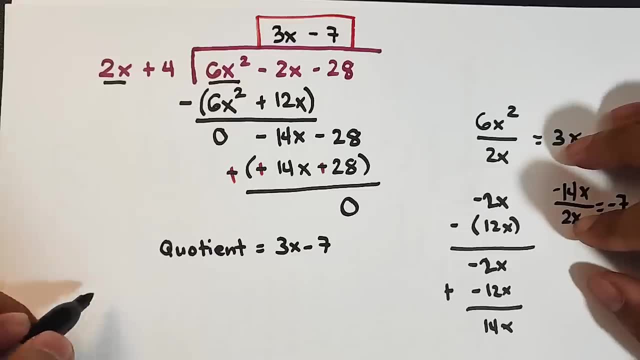 The quotient is equal to 3x minus 7, or what natin gawin dito is that we have 6x square minus 2x minus 28. divided by 2x plus 4 is equal to 3x. 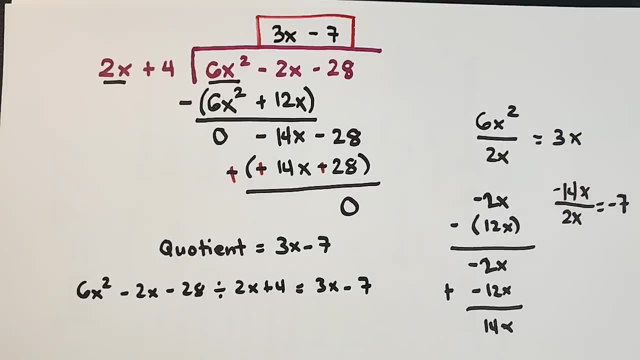 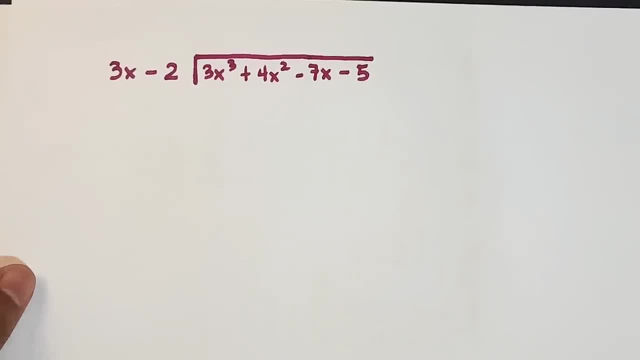 minus 7.. And that's it, guys. So let's continue solving the next problem. Okay, let's have another problem. For the next problem, same rotation: divide the leading terms, multiply and then subtract. Let's try. 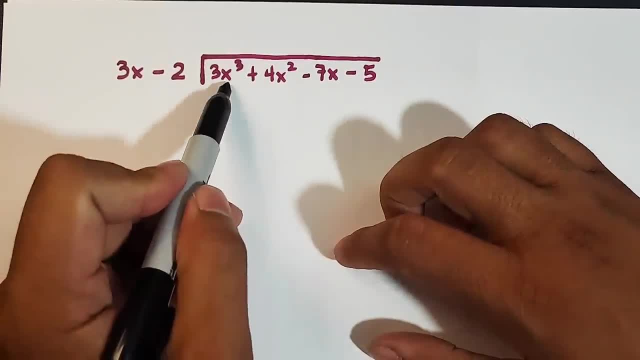 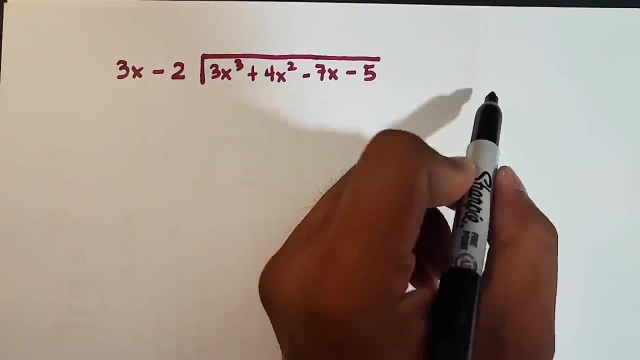 Okay, So let's try this one, eh, Leading term. leading term: 3x cubed divided by 3x. So lagyan natin dito para meron kayong side solution: 3x cubed divided by 3x. 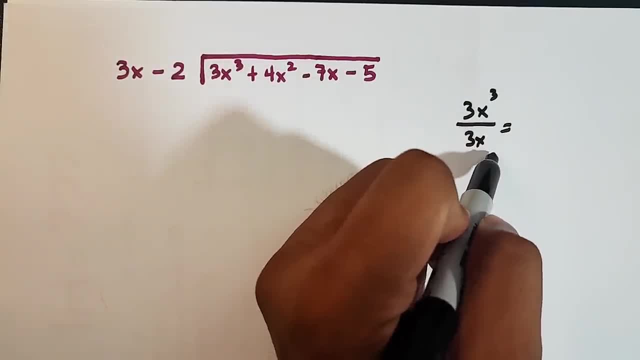 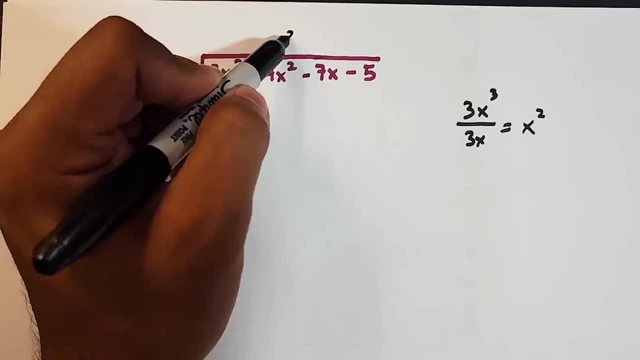 So 3 over 3 is 1.. x cubed over x is x squared. So nagyan natin, dito is x squared, Dito sa pangalawa. So what's next, sir? Ang next naman natin ito: 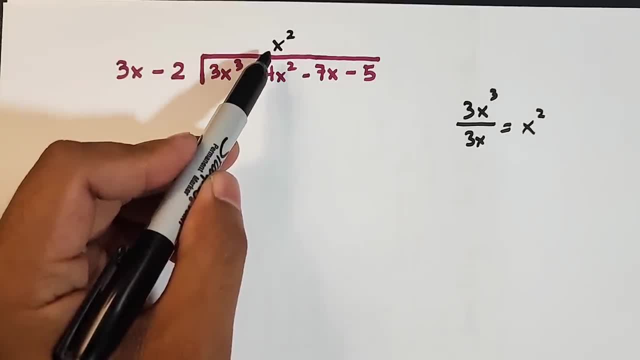 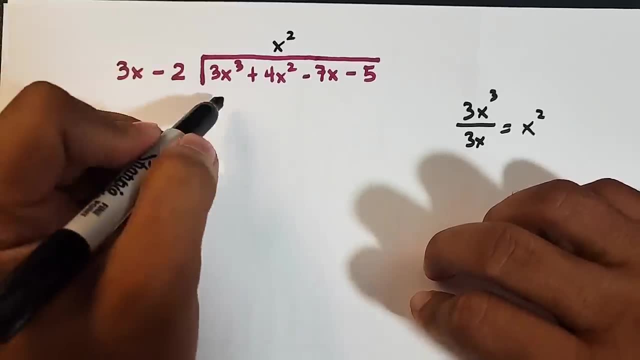 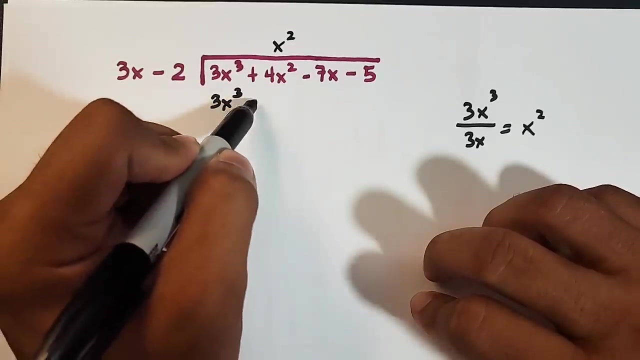 Multiply 1 by 1.. Okay, So multiply natin. It will become this: one x squared times 3x, That is 3x cubed x squared times negative 2x, That is negative 2x squared. 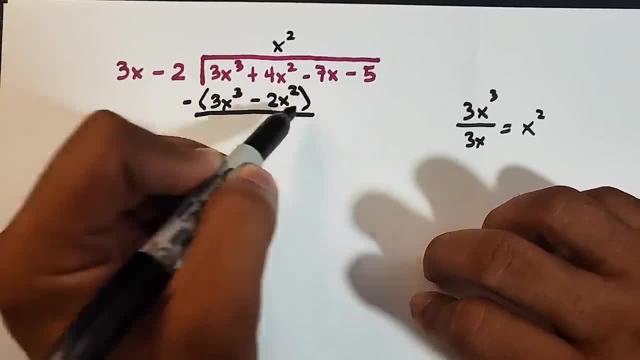 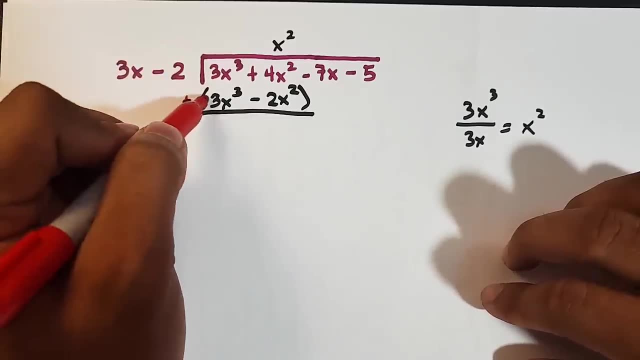 So subtract natin And don't forget na ano siya. i-enclose yun sa parenthesis. Sige, pakita ko sa inyo Magbabago ng sign. ito Magiging addition, ito, Ito magiging. 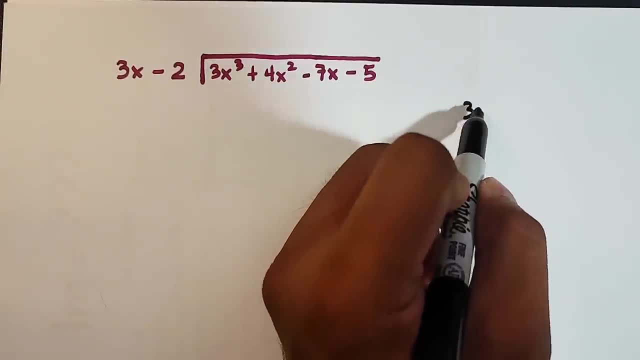 So let's put it here. So you have a side solution: 3x cubed divided by 3x. So 3 over 3 is 1.. x cubed over x is x squared. So what we put here is x squared. 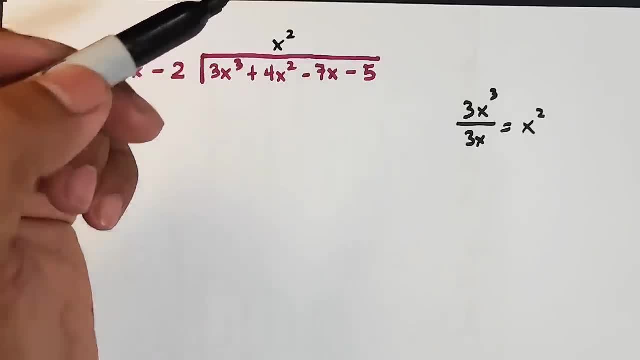 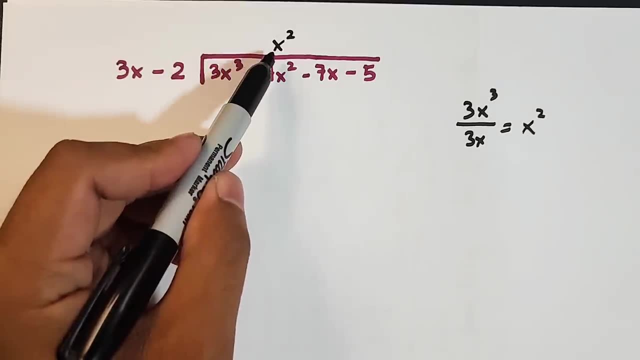 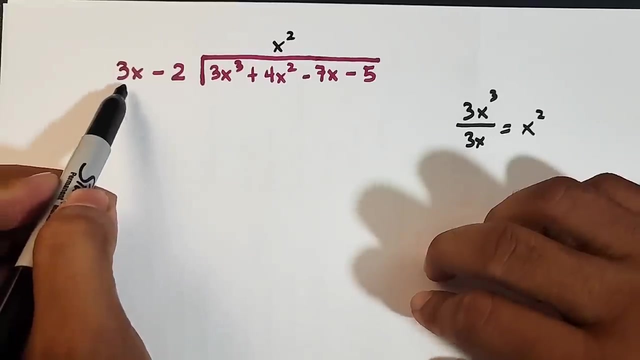 This is the second one. So what's next, sir? What's next is this: Multiply 1 by 1.. Okay, So let's multiply. It will become this: one x squared times 3x, That is 3x cubed. 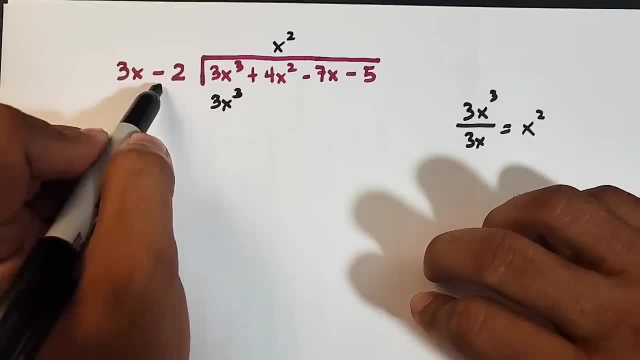 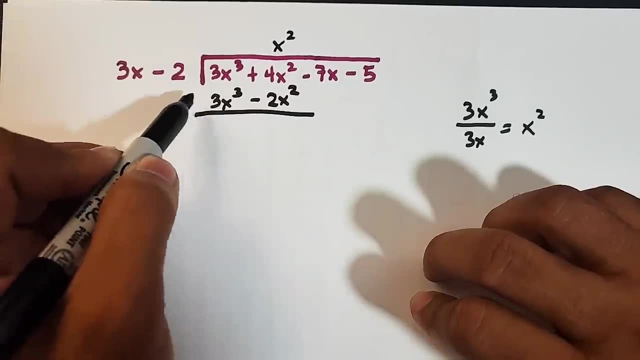 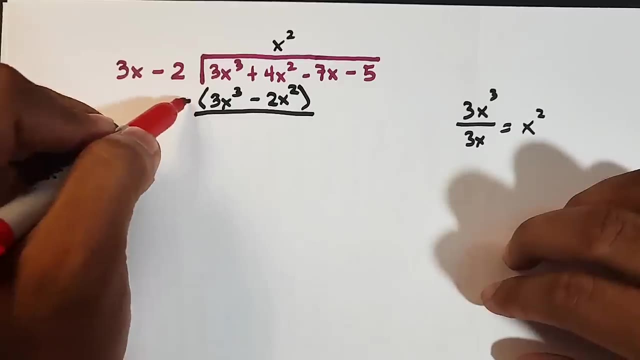 x squared, minus times negative 2x. That is negative 2x squared. So let's subtract And don't forget that it's in the parenthesis. Okay, Let me show you. The sign will change. This will be addition. This will be subtraction. 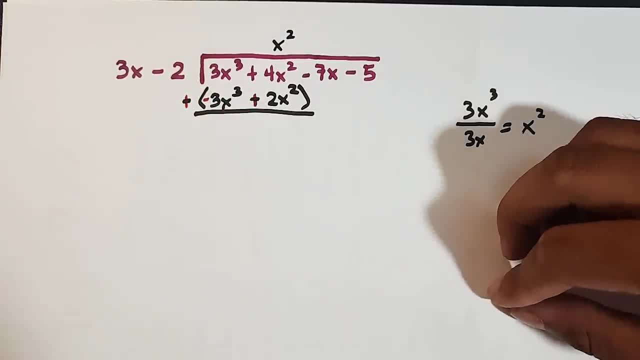 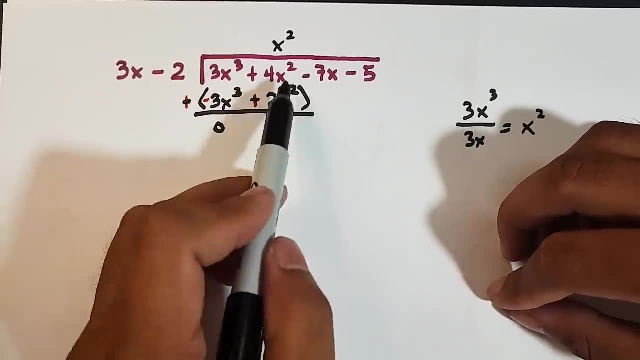 Or negative. This will be positive. So what will happen is that we have now 3x cubed plus negative 3x. It will become 0.. This is 0.. This is 0.. This is 4x squared plus positive 2x squared. 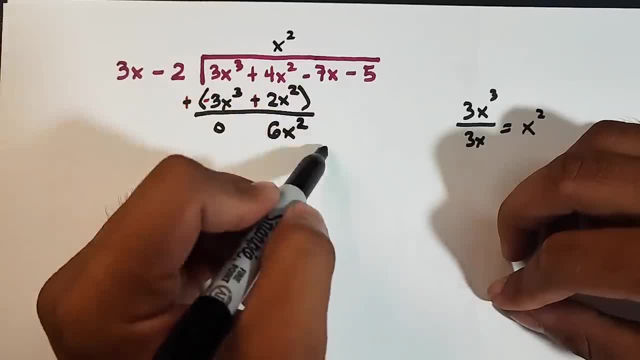 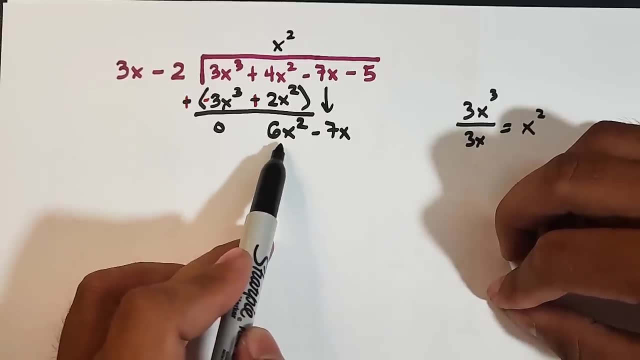 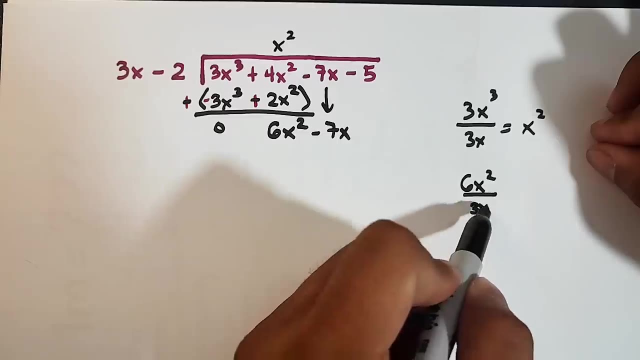 That is equal to 6x squared. Then bring down- Let's do it one by one- Negative 7x. So this is your new leading coefficient: 6x squared divided by 3x. So 6 divided by 3 is 2.. 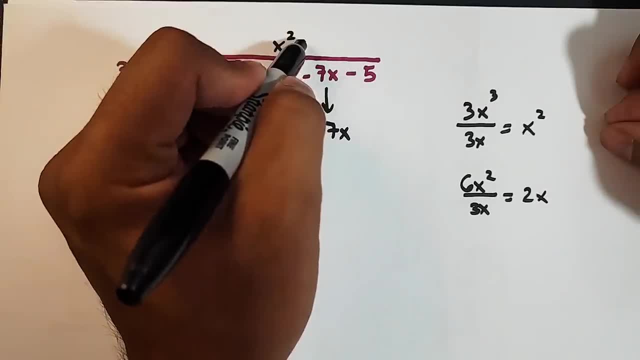 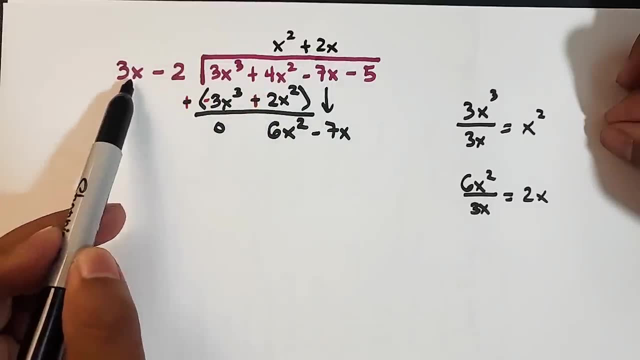 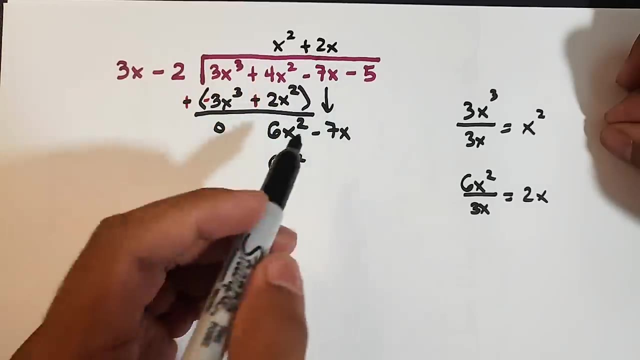 x squared, divided by x is x. So this is it. Put it here: Plus 2x Multiply 2x times 3x is 6x squared, 2x times negative 2 is minus 4x Subtract. 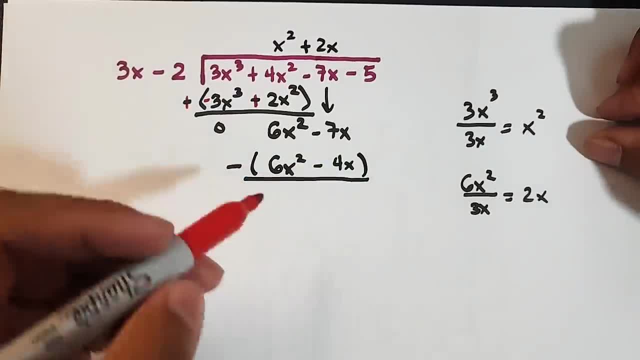 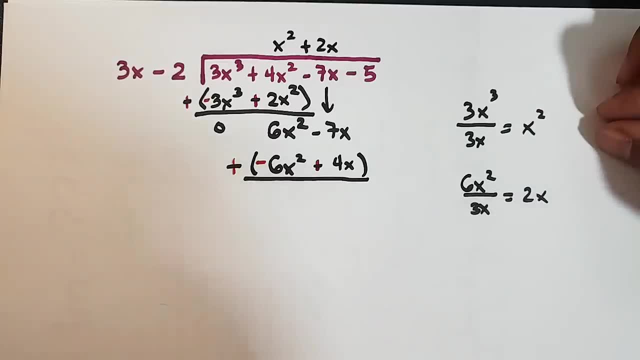 Then in close, by parenthesis, Change the operation Plus. This will be negative, This will be positive. So what will happen? 6x squared plus negative, 6x squared, That will be 0 again. guys, Negative 7x plus positive 7x. 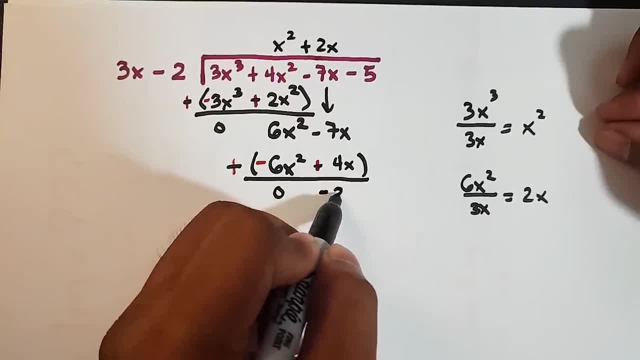 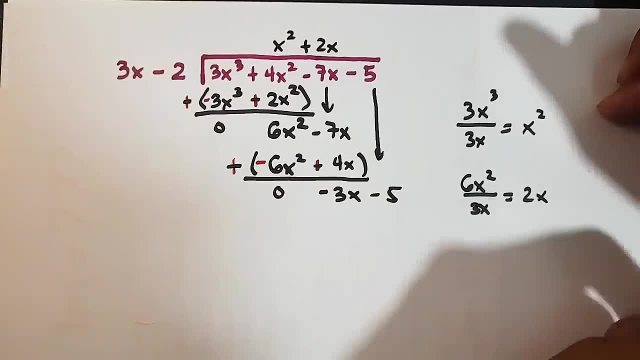 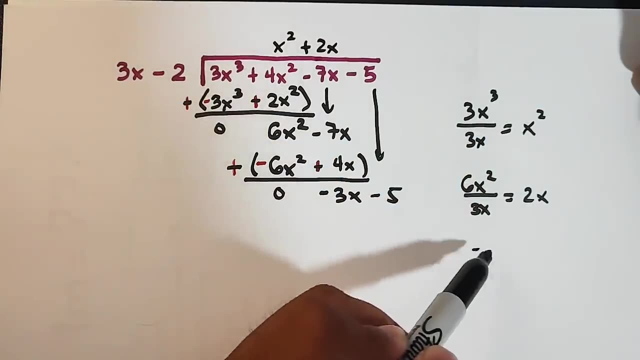 That is Positive 4x. That is negative 3x. Then bring down this last one, which is negative 5. Divide again our leading coefficient. We have- We are here in this part- We have negative 3x over 3x. 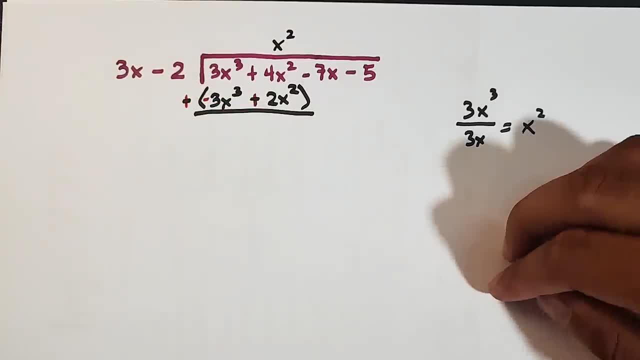 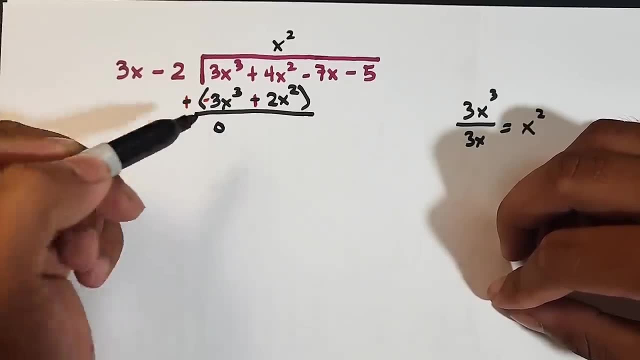 subtraction or negative Ito magiging positive. So what will happen is that we have na 3x cubed plus negative 3x Magiging. zero na yan guys. Zero dito, Zero Ito naman. 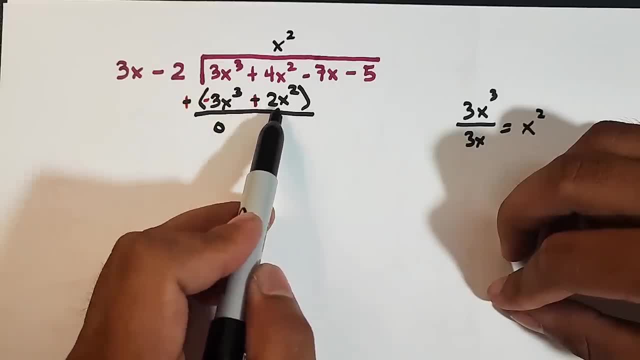 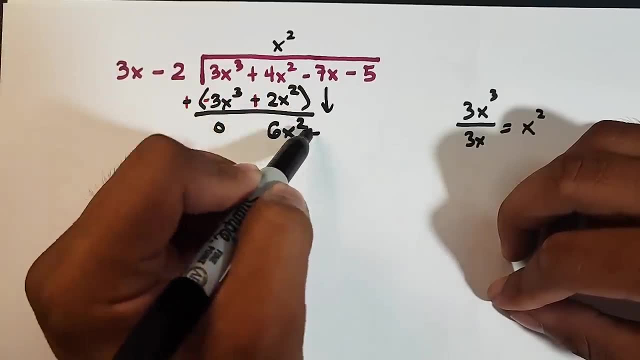 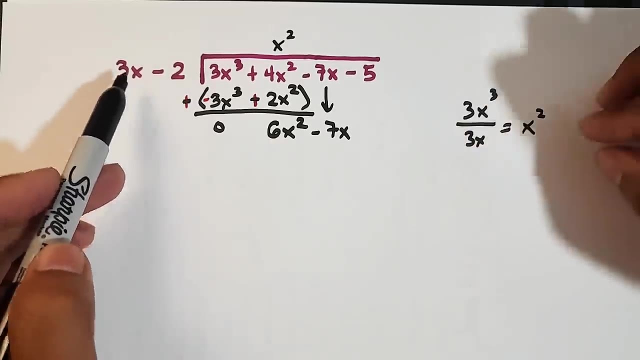 4x squared plus positive 2x squared, that is equal to 6x squared. Then bring down Paisa, isa tayo, ah, Negative 7x. So tanong yung panibagong leading coefficient mo: 6x squared divided by 3x. 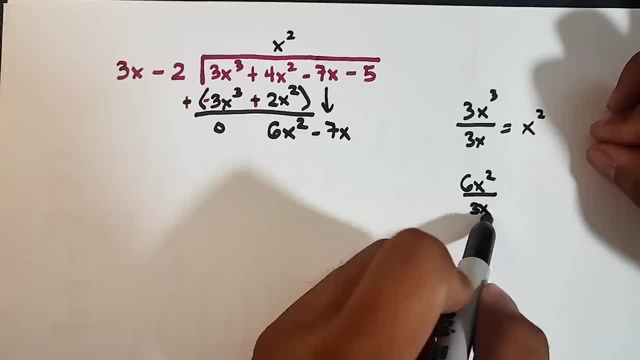 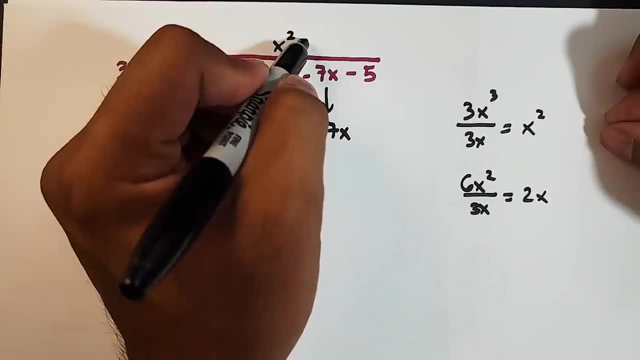 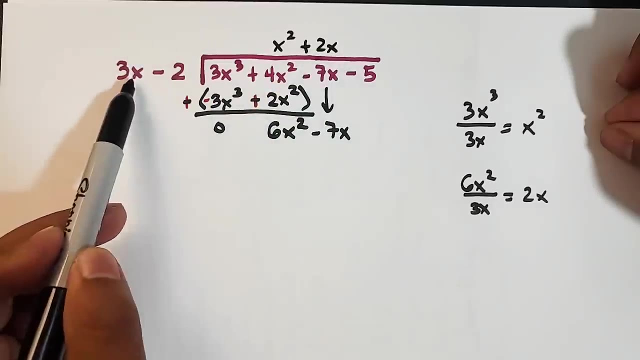 So 6x squared divided by 3x. So 6 divided by 3 is 2.. x squared divided by x is x. So ito na siya, Lagyan mo dito plus 2x. Multiply 2x times 3x. 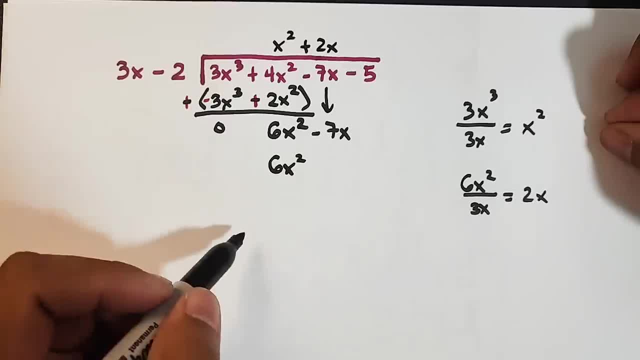 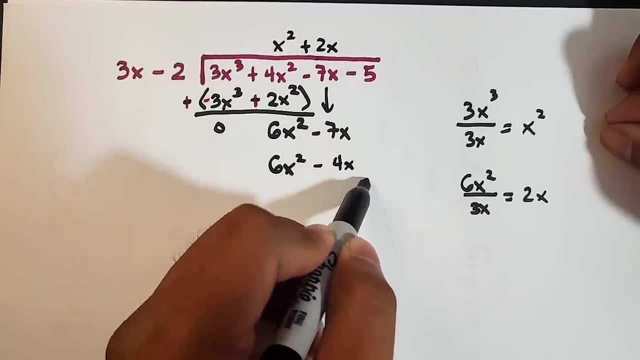 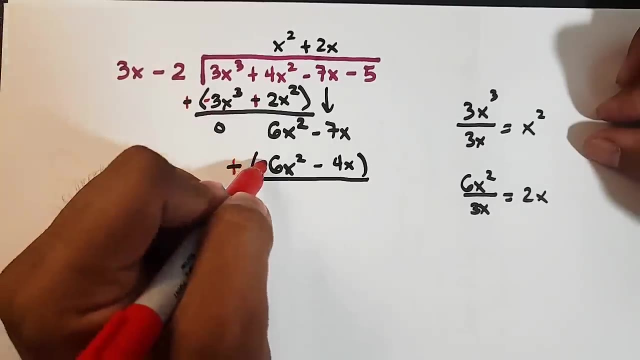 is 6x squared 2x times negative, 2 is minus 4x Yan Subtract Then enclose by parenthesis: Change tayo ng operation Plus. Ito magiging negative, Ito magiging positive. 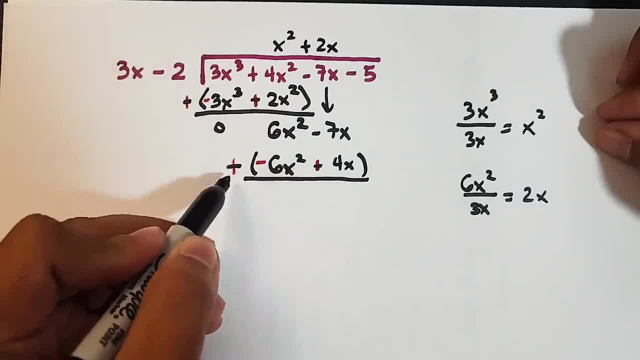 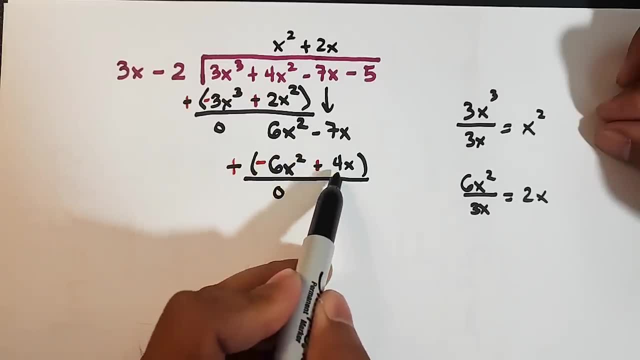 So what will happen? 6x squared plus negative, 6x squared, Magiging zero ulian guys. Negative 7x plus positive 7x. That is, ah, positive 4x. That is negative 3x. Then bring down itong. 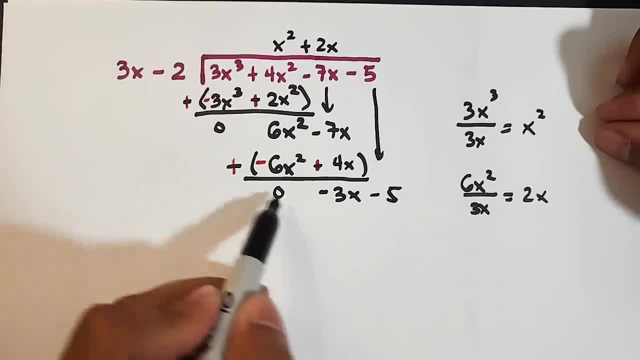 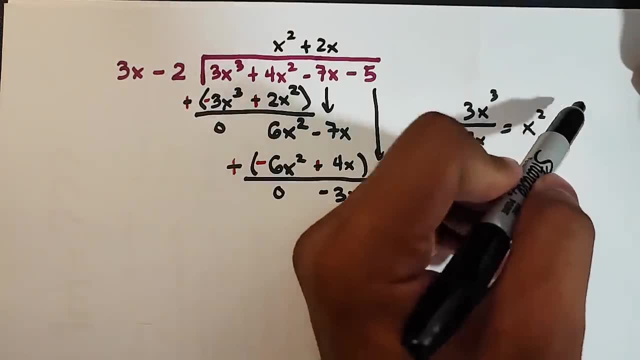 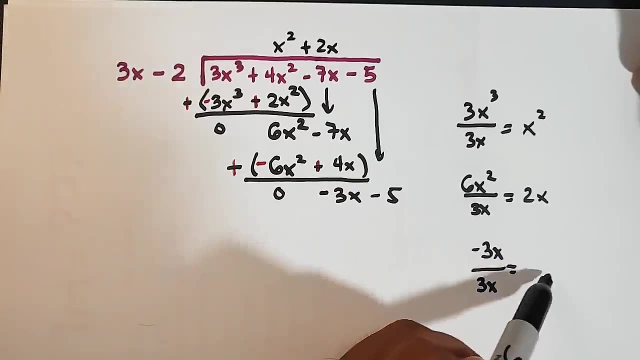 last one natin, which is negative 5. Divide ulit yung ating leading coefficient. We have dito na tayo, sa part na to, We have negative 3x over 3x. That is definitely negative 1. So dito lagyan natin. 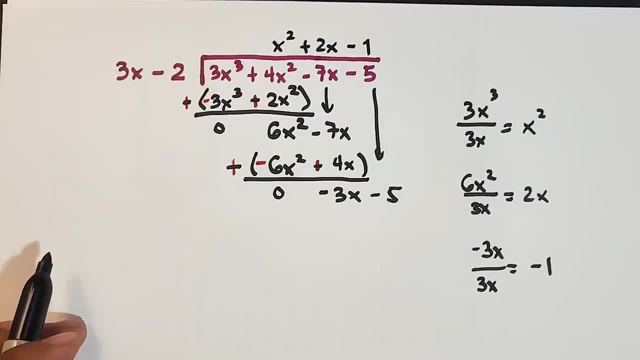 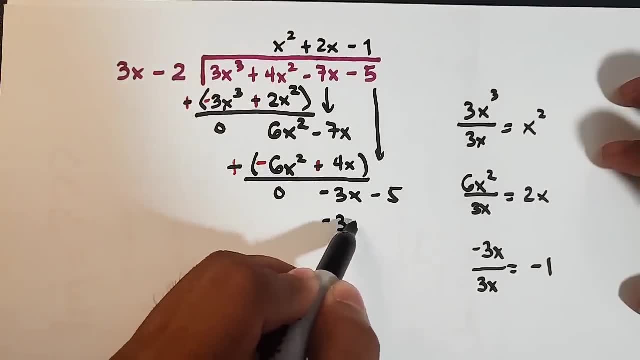 minus 1.. Okay, So what will happen? It's this: Multiply natin Negative 1 times 3x. That is negative, 3x. Negative 1 times negative: 2.. That is positive 2.. 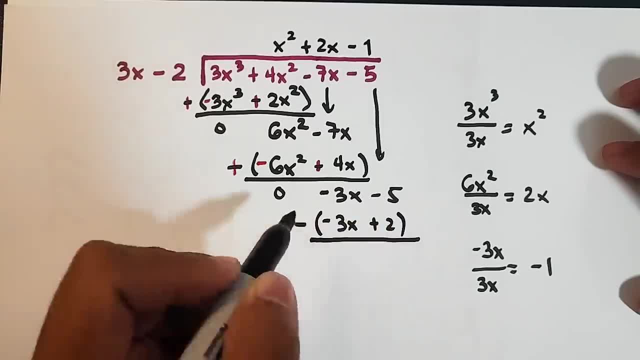 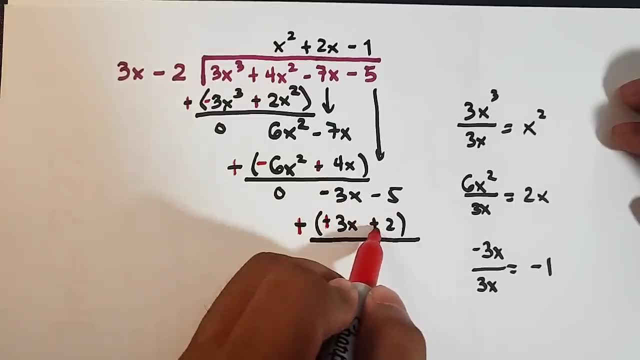 Okay, Subtract ulit. natin Enclose by parenthesis Tandaan babagay natin yung operation Plus Itong negative natin magiging positive, Itong positive natin magiging negative. So what will happen is this: 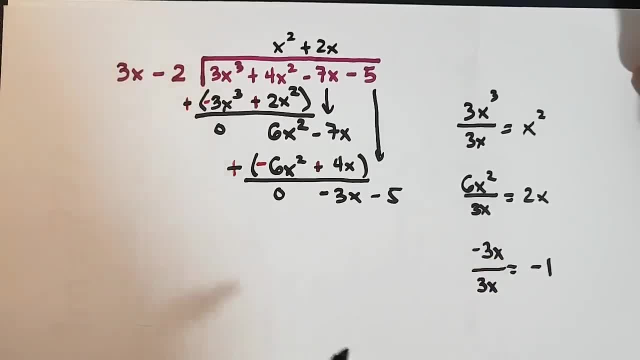 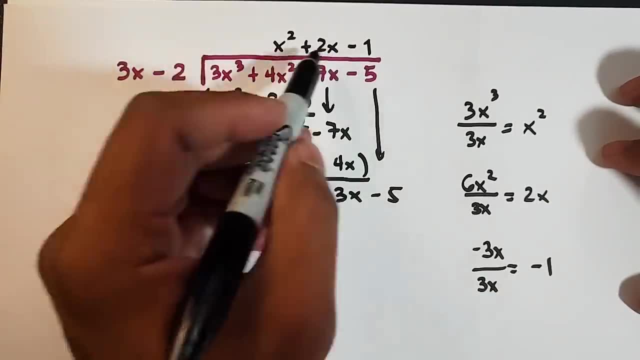 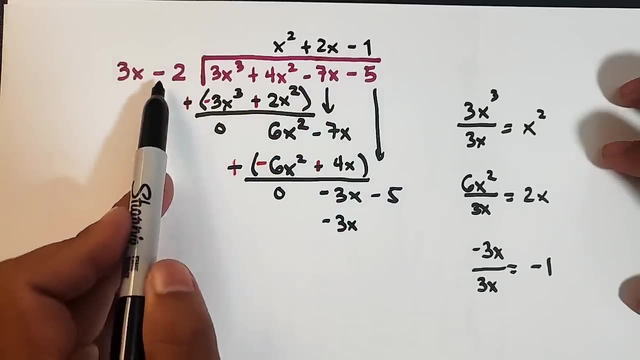 That is definitely negative: 1. So here we put minus 1. Okay, So what will happen is this: Multiply Negative 1 times 3x. That is negative. 3x Negative 1. Times negative 2. That is positive 2.. 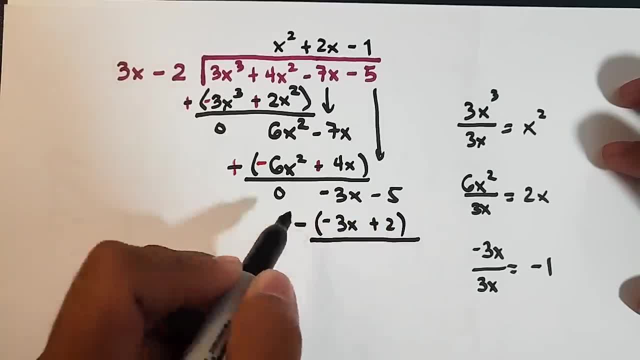 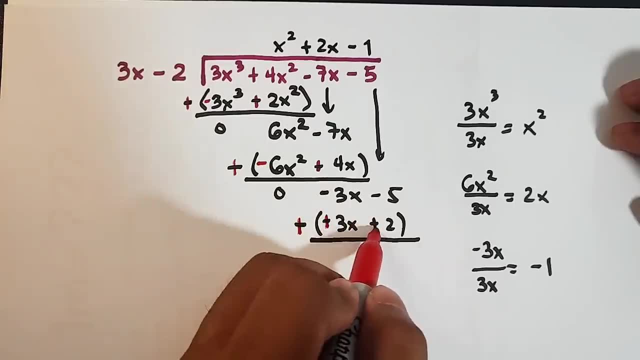 Okay, Subtract again In close, by parenthesis, Remember We will change the operation Plus, This negative will be positive, This positive will be negative. So what will happen is this: Negative 3x plus 3x, That is 0 again. 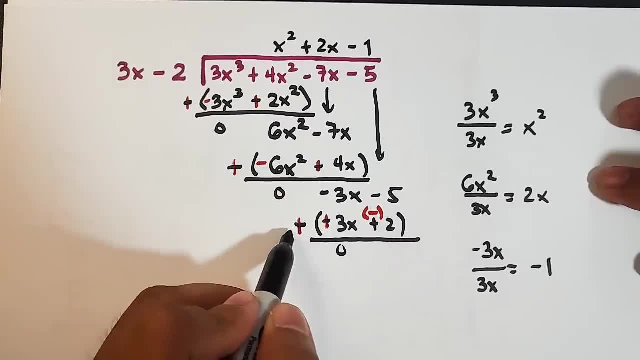 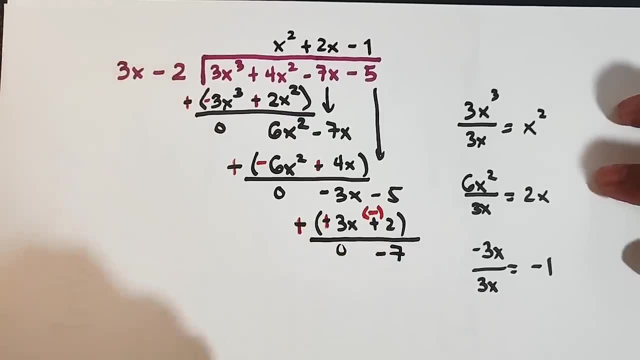 That is 0.. Negative 5.. 5 plus okay, plus negative 2 na yan, that is negative 7.. Ito yung magiging remainder natin. So paano ngayon natin sulit yung sagot natin. 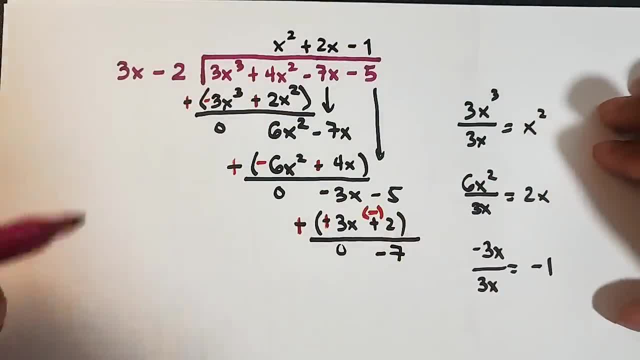 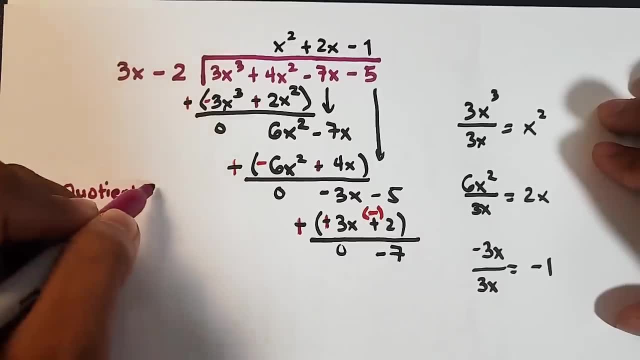 Mayroon ba yung format guys? Ito yung magiging format natin. ha, Ang format natin is quotient, Tapos positive, negative, Kasi ano to ginagamit yung format ito kapag mayroong remainder. 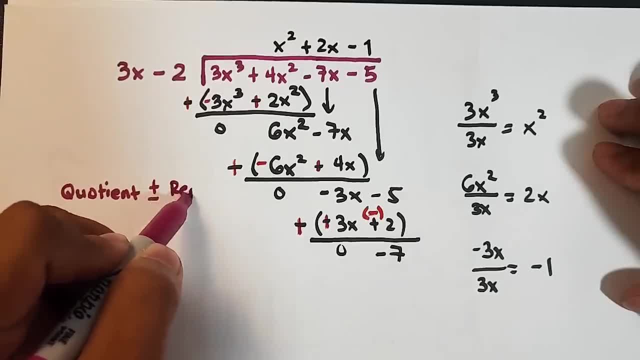 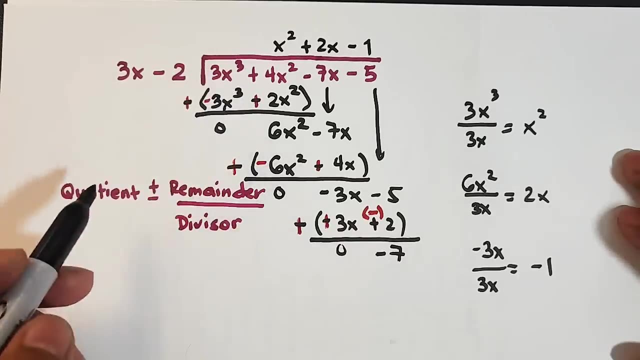 Quotient positive, negative remainder over divisor. So to express our final answer, ganito ang gagawin nyo guys. Okay, Copy natin yung ating divisor: 3x cubed plus 4x squared minus 7x minus 5.. 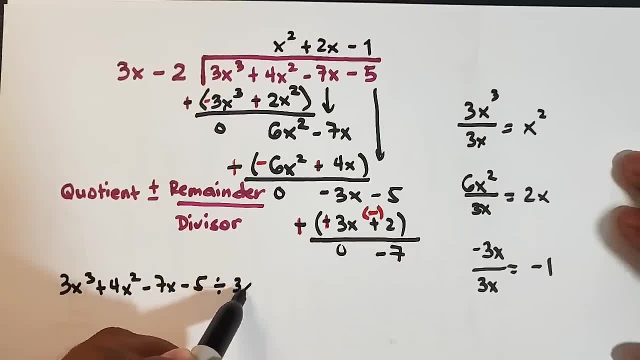 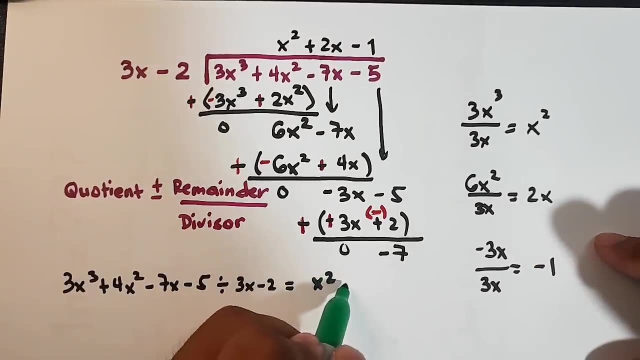 Divided by 3x minus 2 is equal to ito na Follow natin ito, Copy muna natin yung quotient. Yung quotient natin is gamitin yung ibang kulay: X squared plus 2x. 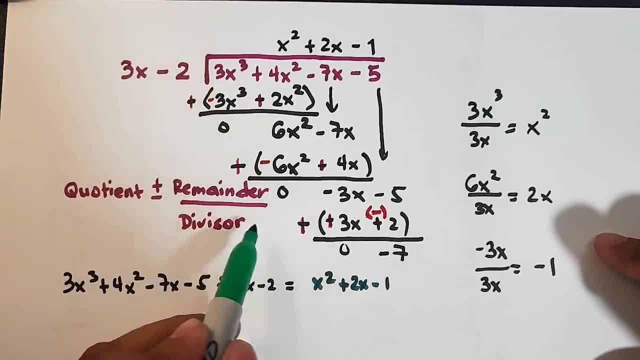 Kasi baka hindi alapin sa inyo ito minus 1.. Ito na Remainder muna. Since yung remainder natin is negative, magiging negative 7.. Over your divisor, that is 3x minus 2.. 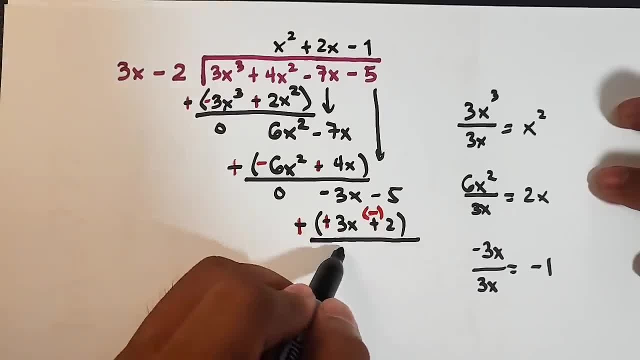 Negative 3x plus 3x, That is 0.. Zero na yan, Zero Negative 5 plus okay plus negative 2 na yan, That is negative 7.. Ito yung magiging remainder natin. So paano ngayon natin? 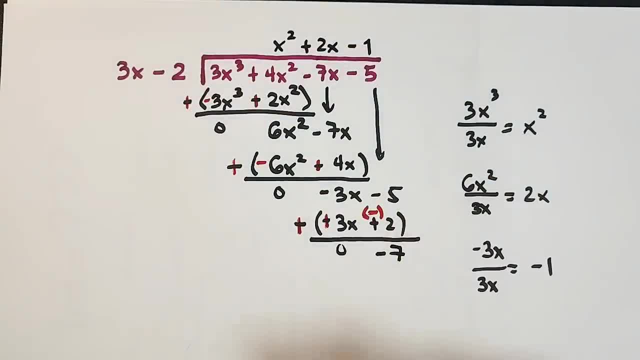 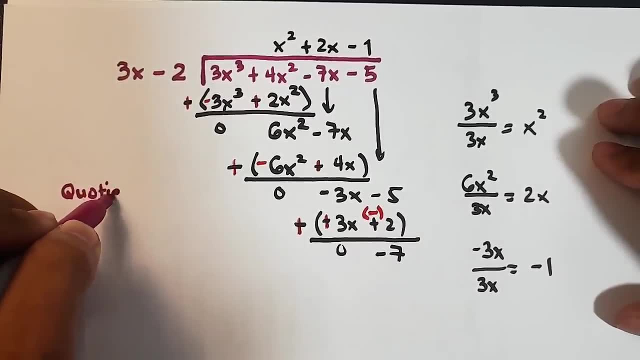 sulit yung sagot natin. Mayroon ba yung format guys? Ito yung magiging format natin. ha, Ang format natin is quotient, Tapos positive, negative, Kasi ano ito. 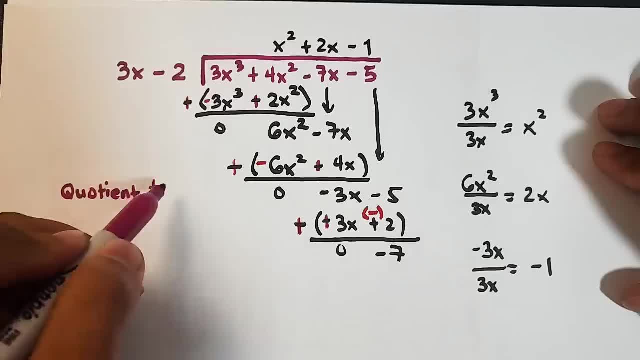 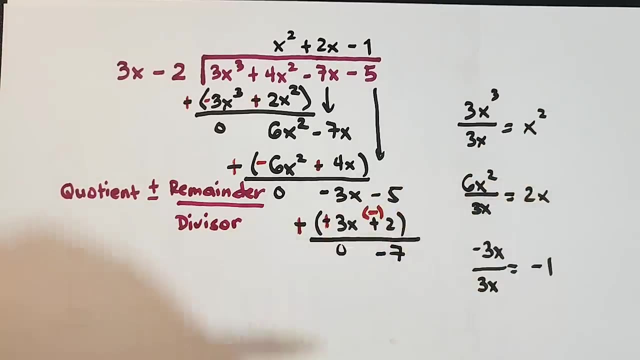 ginagamit yung format ito kapag mayroong remainder Quotient positive, negative, remainder over divisor. So text process or final answer: ganito ang gagawin nyo guys. Okay, Copy natin yung ating. 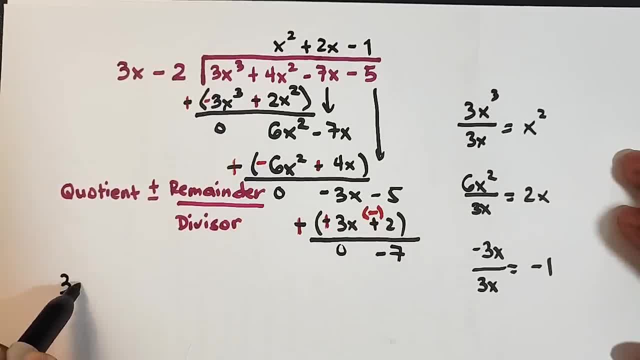 divisor: 3x cube plus 4x square Minus 7x minus 5, divided by 3x minus 2 is equal to Ito na Follow natin ito. Copy mo na natin yung quotient. 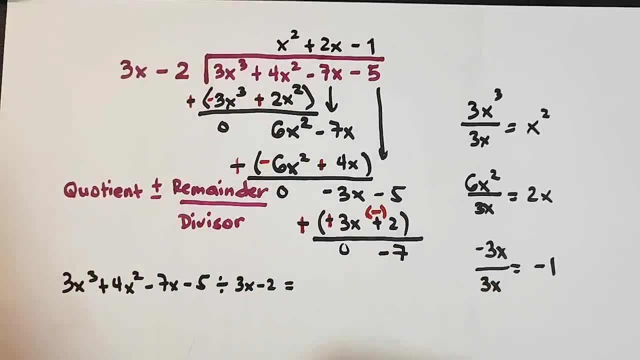 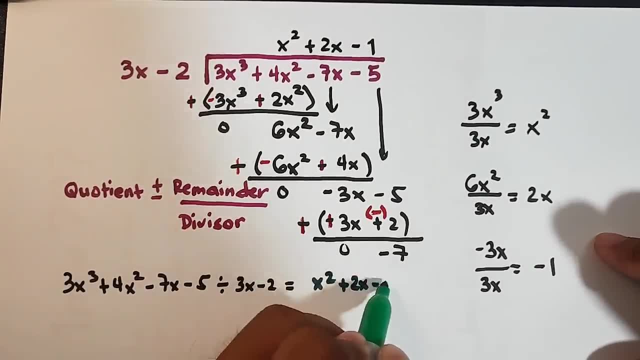 Yung quotient natin is gamitin yung ibang kulay, X square plus 2x, Kasi baka hindi anapin sa inyo ito minus 1.. Ito na Remainder muna, Since yung remainder natin is: 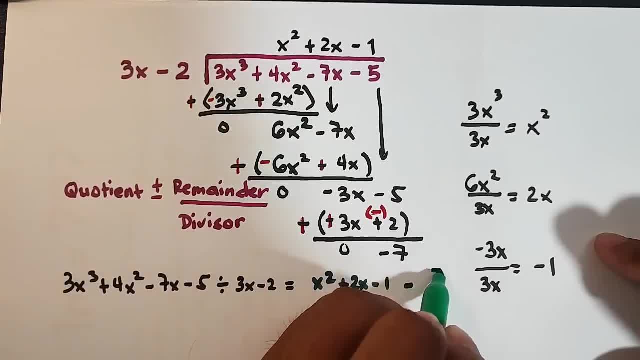 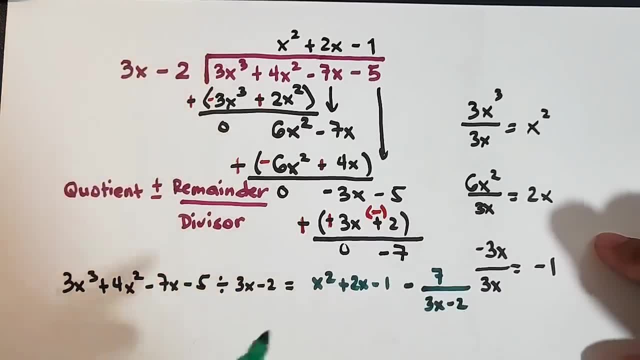 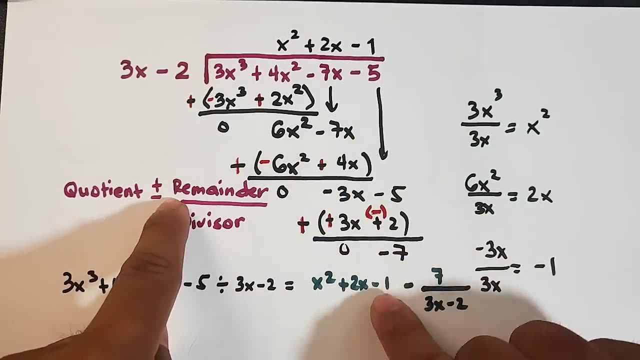 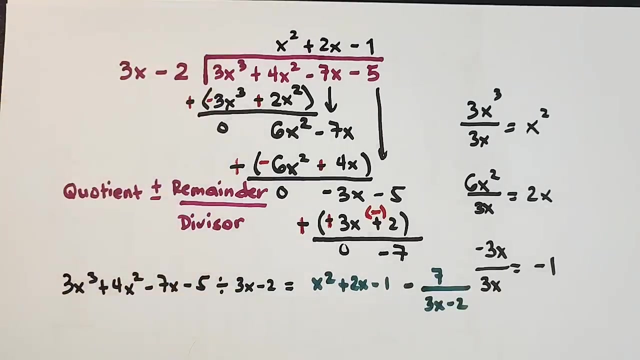 negative, magiging negative 7 over your divisor, that is 3x minus 2.. So, again, quotient ito, since negative, yung ating remainder minus 7 over your divisor, which is 3x minus 2.. So I hope, guys, you learned something from this video. 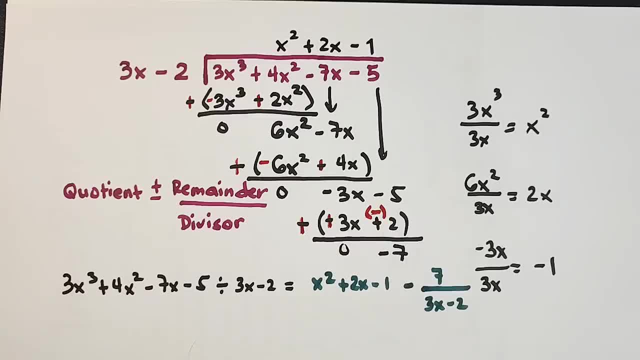 on how to do the long division in dividing polynomials. So if you're new to my channel, don't forget to like and subscribe, but hit mo na rin yung bell button for you to be updated sa ating latest uploads. Again, it's me, Titcher Gon. Maraming, maraming salamat. Bye-bye.